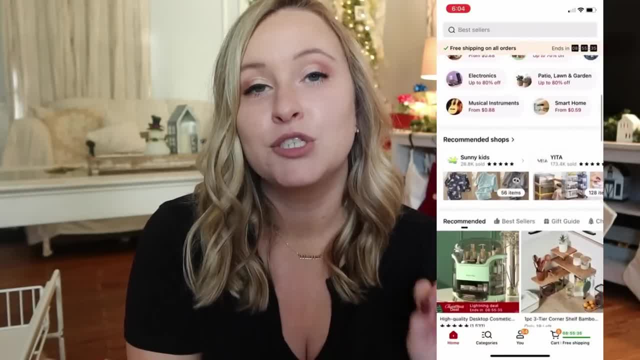 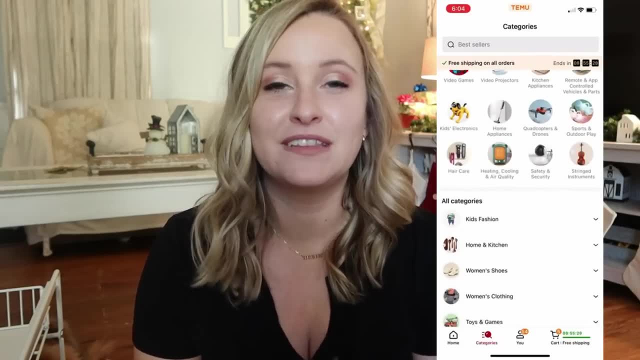 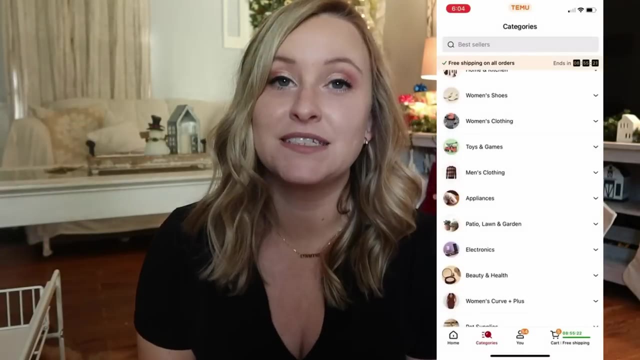 video. So Teemu is a brand new shopping site that offers trendy and top quality products. I foresee a lot of shopping on this app in my future. You can literally shop anything. They have clothing, home decor, kitchen items, all kind of organization things, pet supplies, toys and so much more. 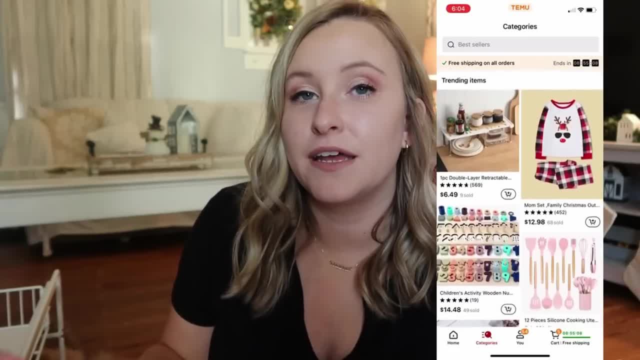 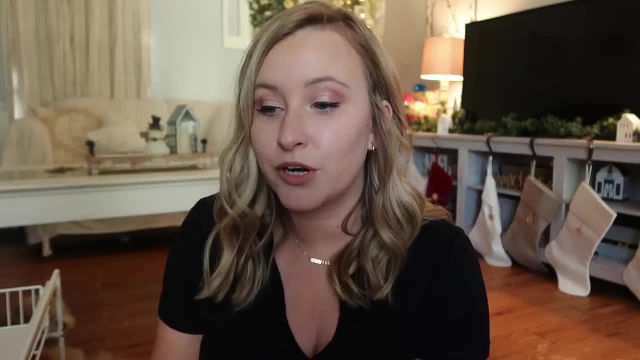 starting at 99 cents. So it's kind of like Amazon, except much lower prices. but I'm going to go ahead and show you guys a haul of everything that I organized. So I'm going to go ahead and show you so you can see the quality of the product. So I'll start with this. I'm really, really excited. 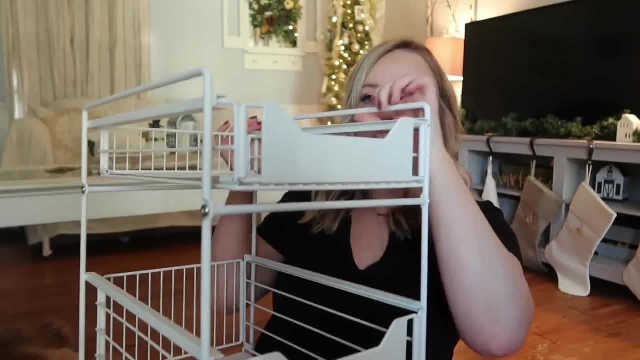 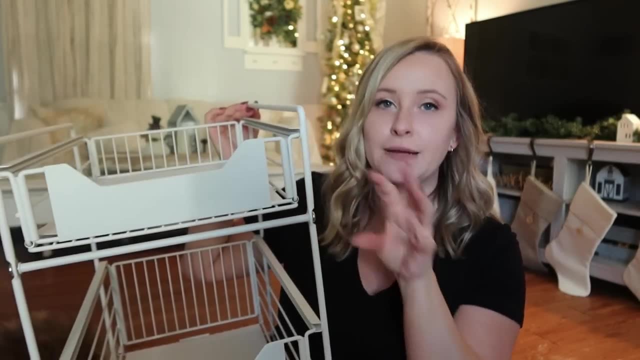 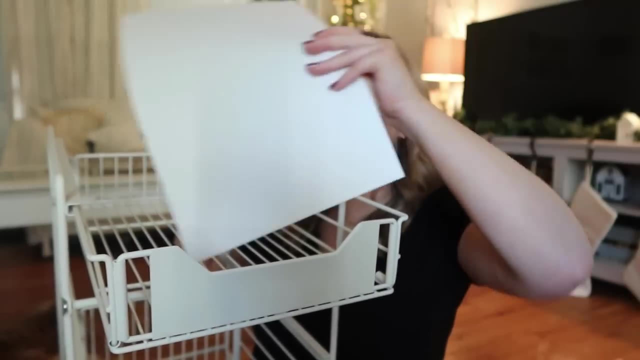 about this thing. So it's like a under the sink organizer- at least that's what I am going to try to use it for. I don't know about how the pipes are laid out, if it's actually gonna work, but it's got two drawers. I really like that. it has these little sheets here that it's like a plastic. 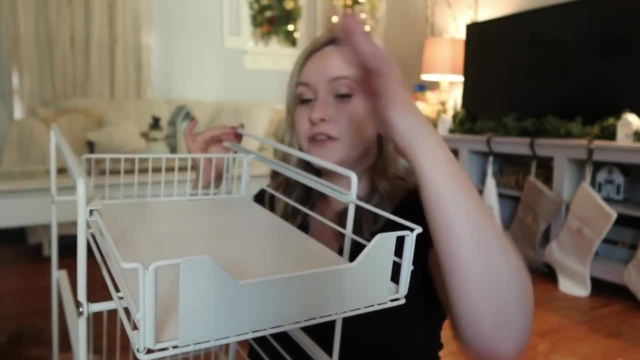 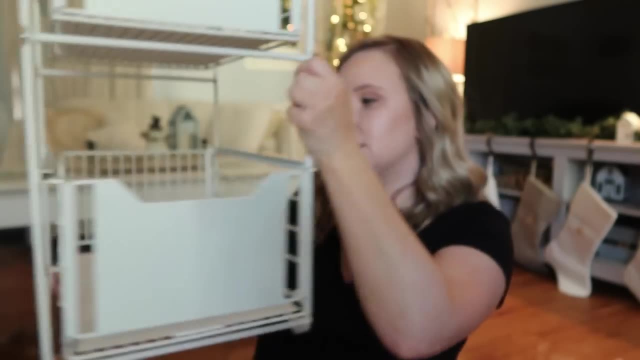 material that you can lay on top of the wire so that your stuff doesn't fall through the drawers. This one on bottom is deeper so I might can put like hairspray and things like that in there. I also got us a new laundry basket, The one that we have in there. 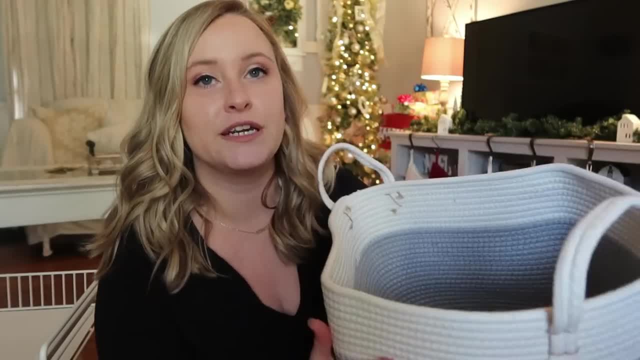 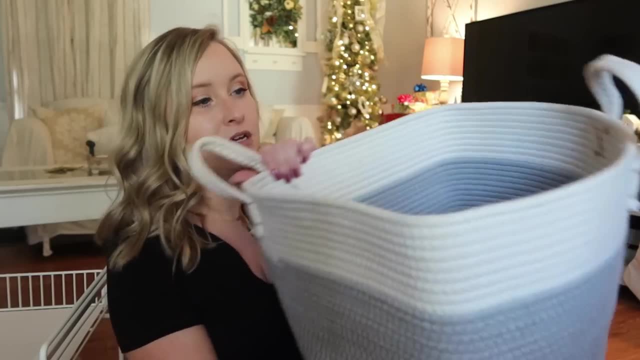 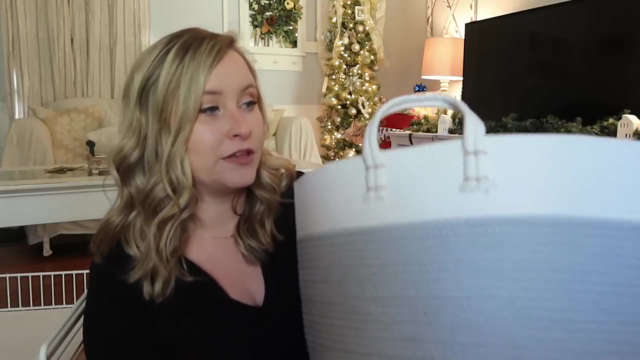 right now is the cheap dollar tree plastic one, and it's kind of falling apart and starting to dry rot. so I wanted to get something like this that we can just throw our laundry into. It's not very big, but the bathroom is not very big either. 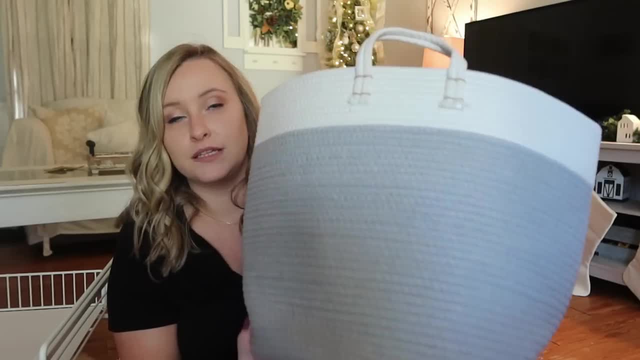 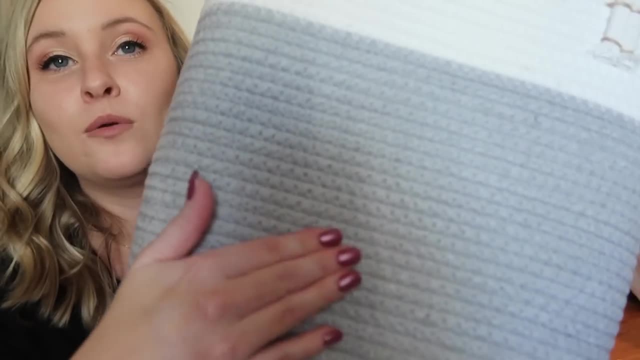 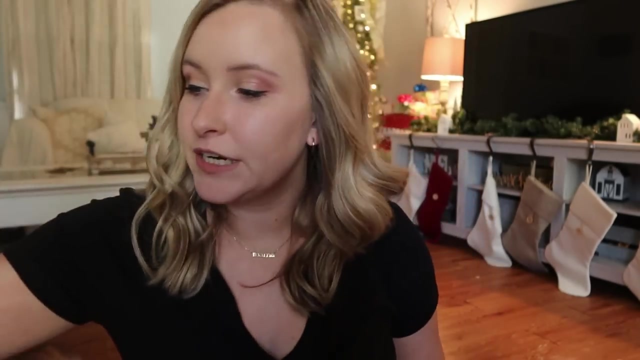 We do a load of laundry every day, so this shouldn't be a problem for this size. but when we take our showers and baths, we can just throw our laundry right in here. I wanted to show you up close. the quality of this is so, so nice, So I think this is going to work perfect for our laundry. 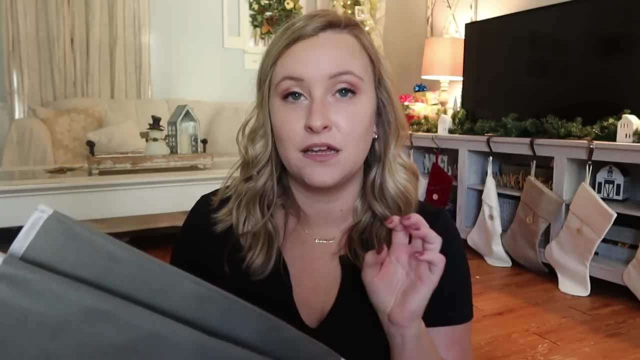 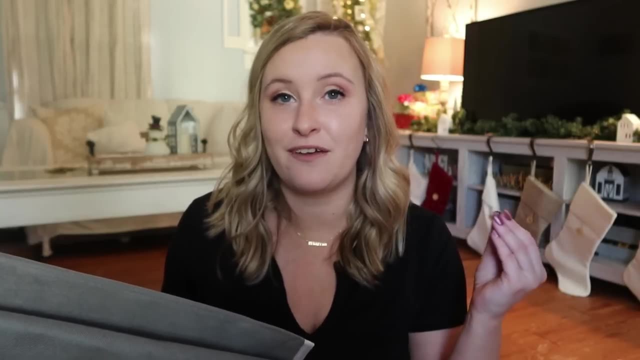 This I am so excited for. This is really going to add some organization space to the bathroom. It's one thing we really struggle with. We don't have a lot of room to put things. We just have under the sink, and then I have that. 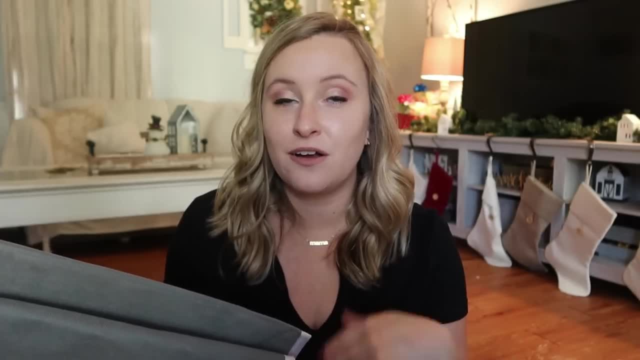 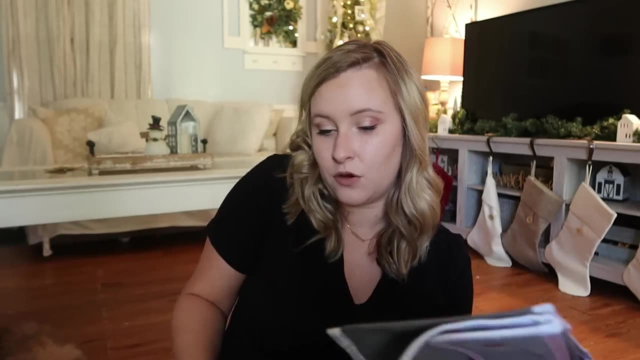 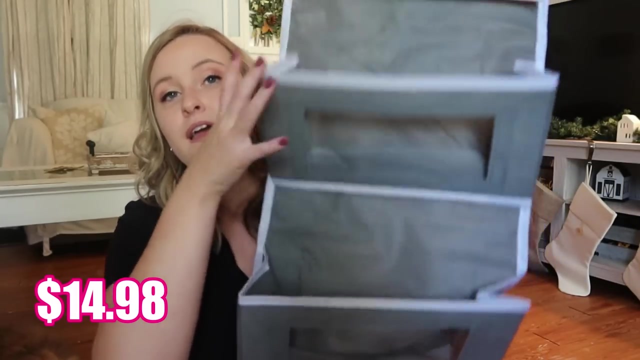 There's a little wire thing next to the sink to put things on, but even that is packed. so I got this. You can hang it over the door and it's got pockets and they're clear so you can see through and know what you are putting in there. 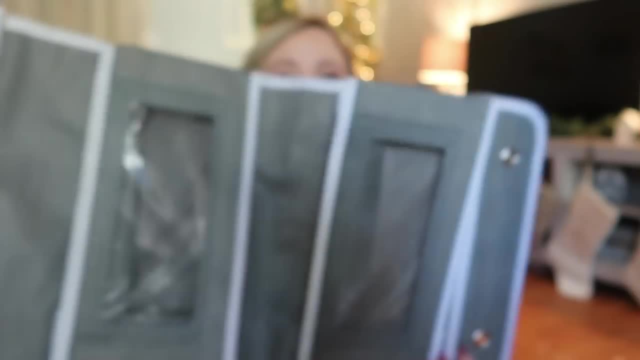 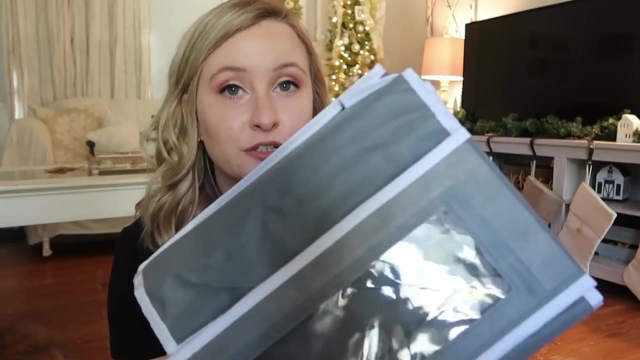 I can put wipes and hair products, all kind of things- in here, So I'm really really excited about this. I think this would be great, also For a baby's nursery. I also got one of these nets to hang up in the shower, maybe for shower. 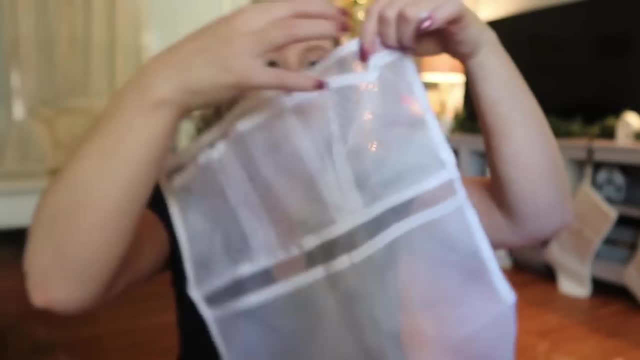 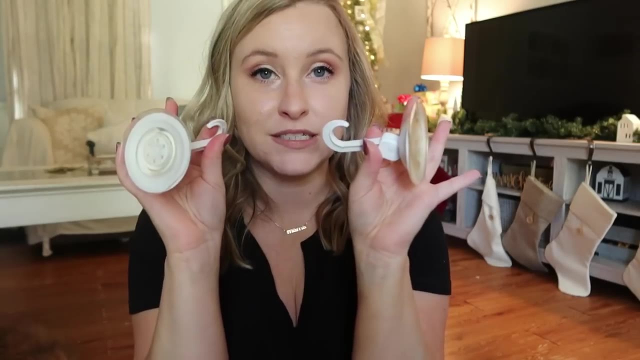 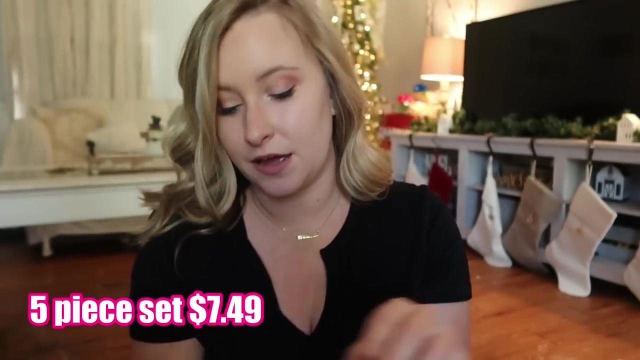 products or bath toys. but it's just a net. It's got three pockets on top and then one larger pocket on the bottom. It comes with two hooks to hang it with. I also picked up some new towel hooks that I can hang onto the wall. Everybody can have a spot to hang their towel. They are really good. 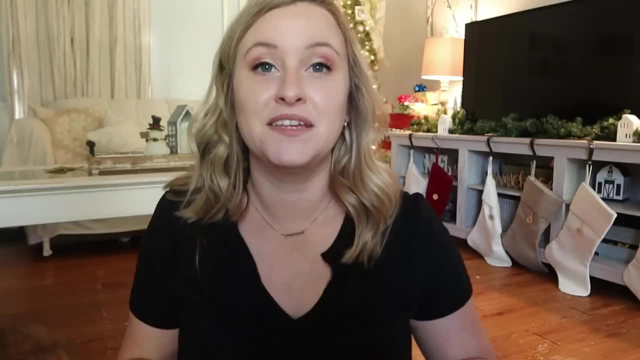 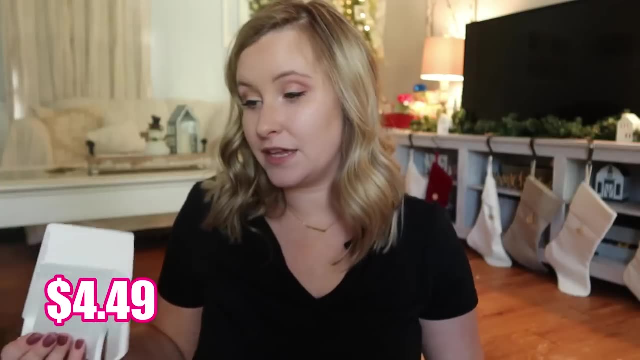 quality. They're just metal. I'm going to show you, guys, how to hang them. I'm going to show you how to hang my towel hooks. Okay, this I got specifically for my blow dryer. I really just want somewhere to be able to hang it. so I got this hanger that I can put up onto the wall and 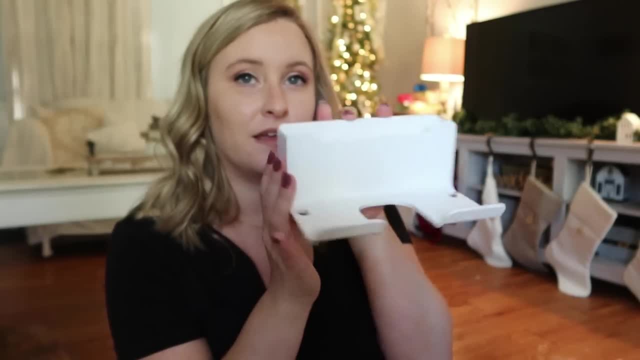 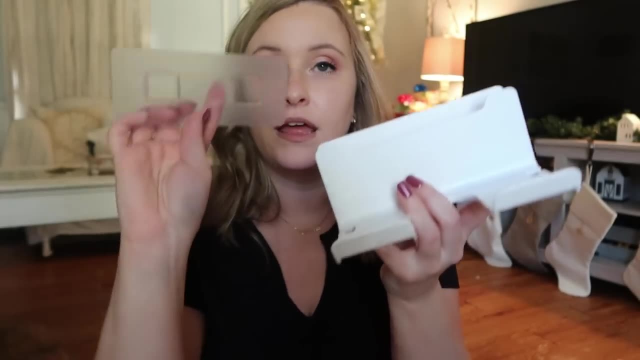 your blow dryer goes in that slot. You sit it sideways and, yeah, you can put other things here in the back of it- Maybe a brush comb, whatever you want- and it comes with a little adhesive thing to stick this onto the wall with These little jars. I got four of these. I was thinking. 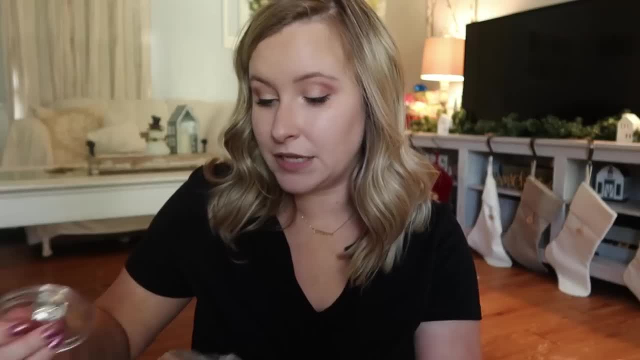 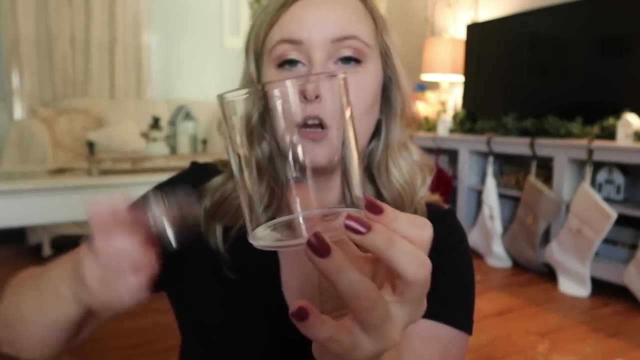 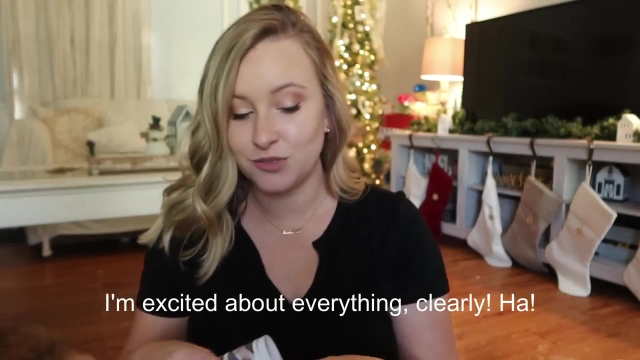 I could put q-tips, cotton balls, maybe some band-aids, floss, anything like that, in here. So they're just little clear jars with lids and there's four of these. Okay, this y'all I am so excited about. I thought this was so, so cute. They actually had a lot of these on the app and I had a. 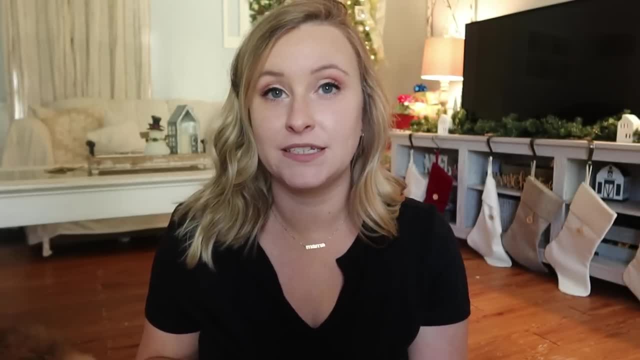 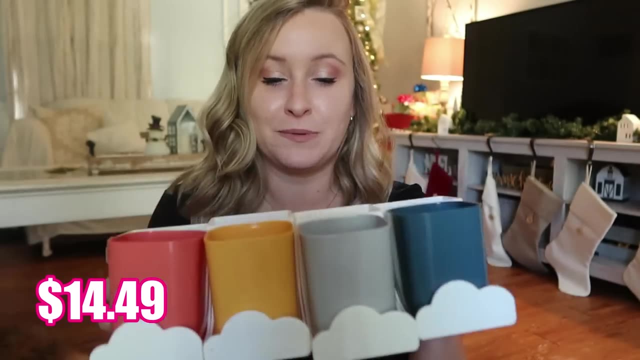 hard time choosing which one I wanted, but this one ultimately ended up being my favorite. So it's in separate pieces right now, but once you get it home it's going to be a little bit more of a. it's all one piece, or supposed to look like. all in peace, Everyone's each individual toothbrush. 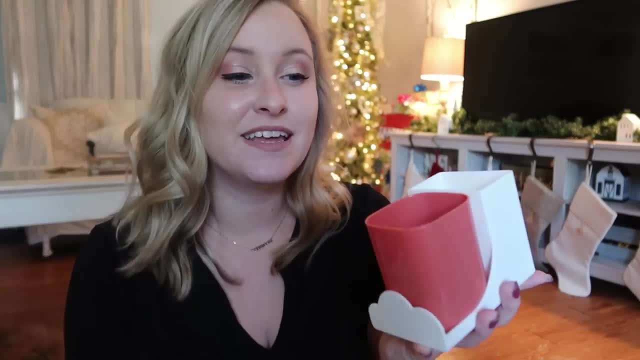 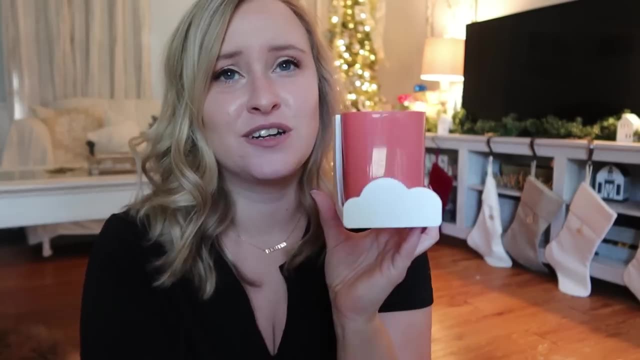 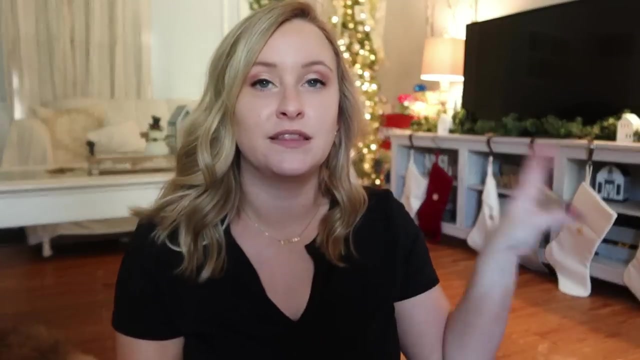 holder with a rinse cup. I love the colors. So basically everyone has their own rinse cup. You can put your toothbrush and toothpaste back here in the back, and I just thought it was so cute. It's little clouds because one problem that we have is that counter space in that bathroom is 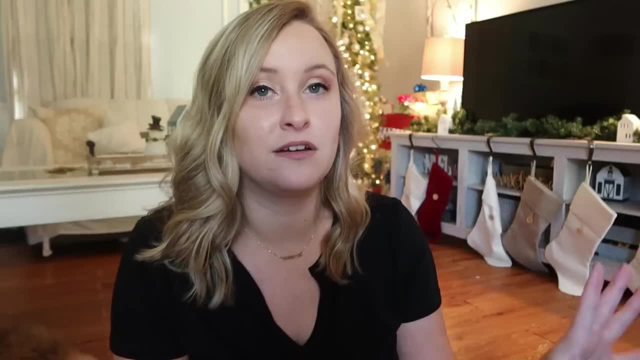 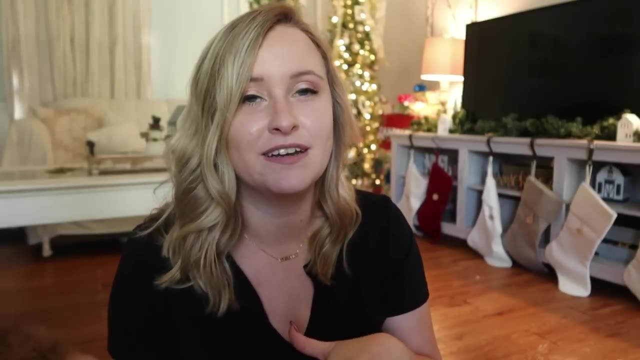 so small. We all have to keep our toothbrushes and toothpaste on the counter and it just it takes up a lot of room and I feel like it's so messy looking. even when we try to straighten it up and make it look neat, it still looks messy. So I'm really excited about these and I think it's going. 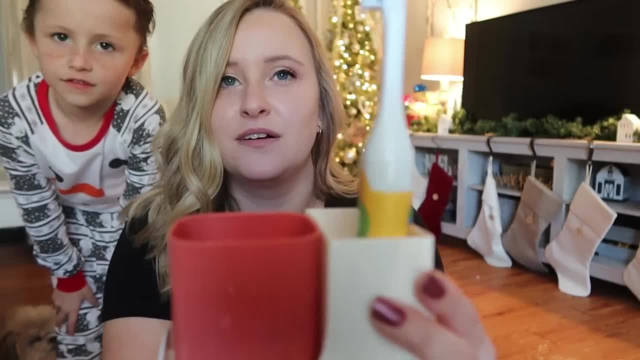 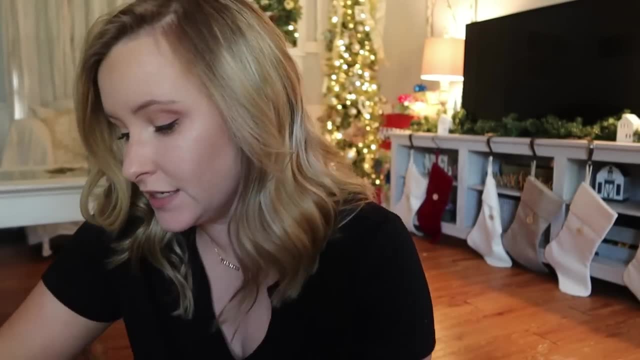 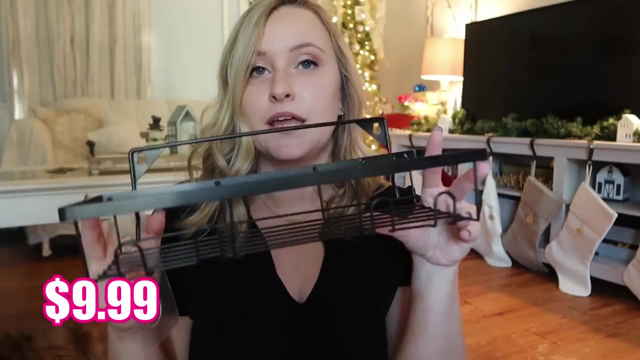 to be really, really cute. Kane wanted to show y'all what it would look like with a toothbrush in the back. It's cute, isn't it? Okay? and then one last thing I got is a new wire shelf. I'm not exactly sure what I'm going to do with this yet. I'm thinking probably in the shower to put some. 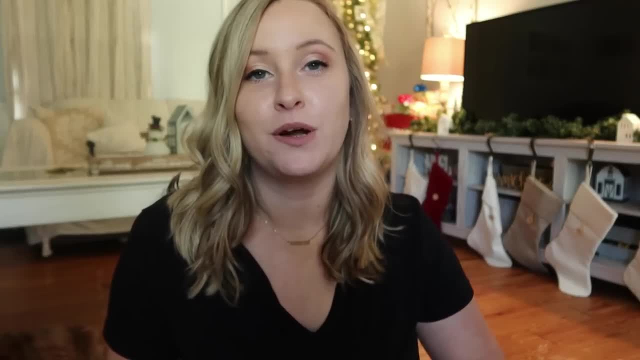 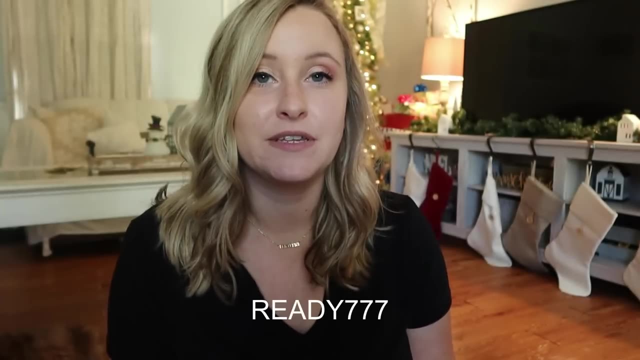 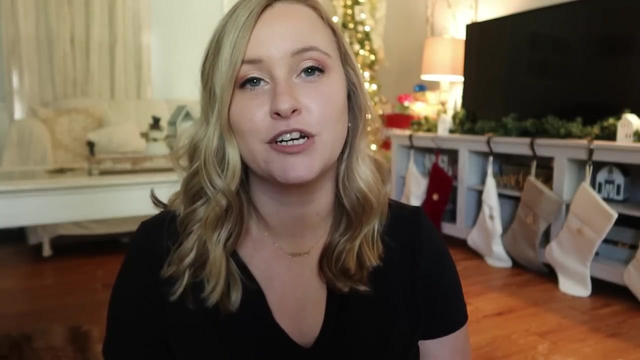 of my shower products. So, because I have teamed up with Timu on this video, my subscribers can get a 30% discount by using my code READY777, or by clicking the link down below in the description box, and Timu offers guaranteed free shipping and free returns within 90 days. So click the link. 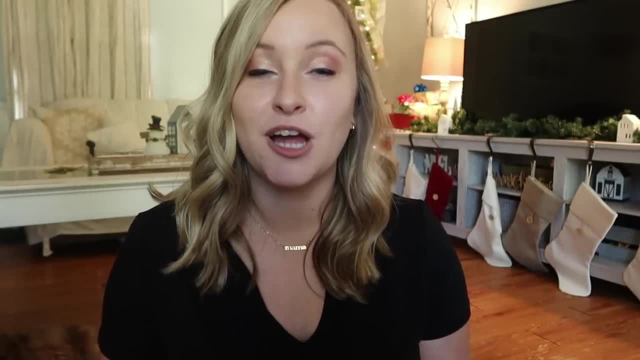 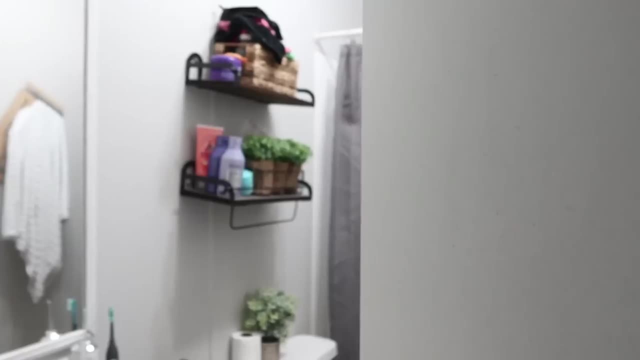 down below in the description box to download and shop the Timu app. Again, a big thank you to Timu for sponsoring today's video. All right, so let's start with the shower. I'm going to start with a before of the bathroom and show you how everything is currently As you. 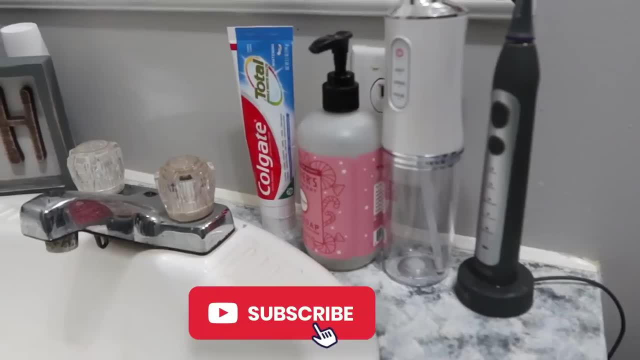 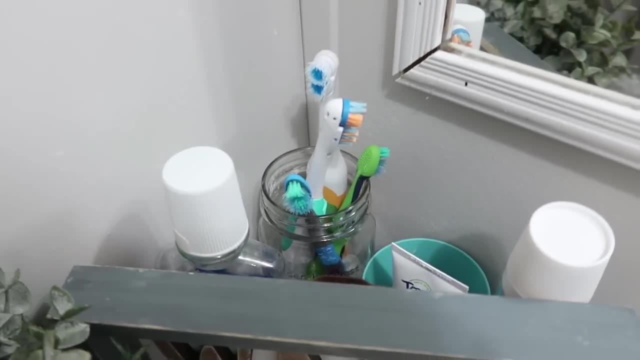 can see, the counter space is little to nothing and right now we have to keep the toothbrushes on the counter because there's just nowhere else to put them. I do try to keep them hidden behind this little wash sign. These over the toilet shelves are packed with so much clutter. 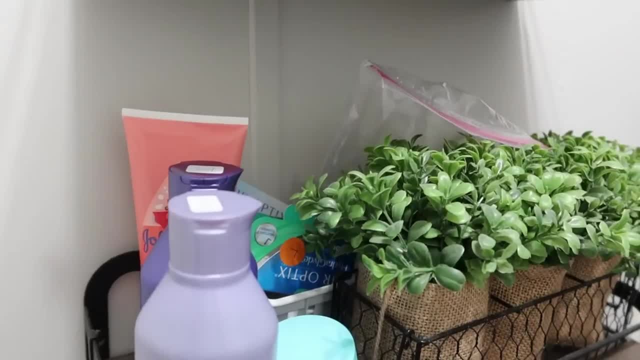 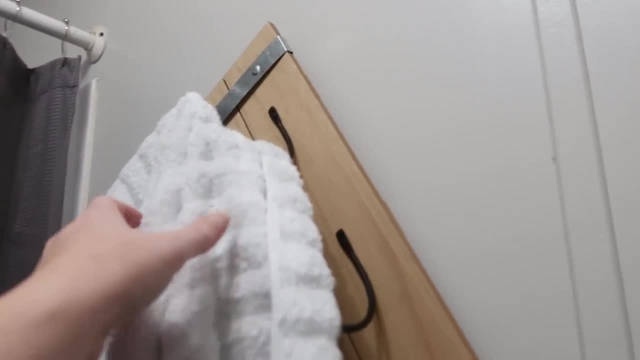 and just not functional at all, so I want to clean those off. today Our towel rack is hanging out. I'm going to start with the shower. Again, by one nail it somehow got knocked down and one of the nails came out, so I'll be fixing that. 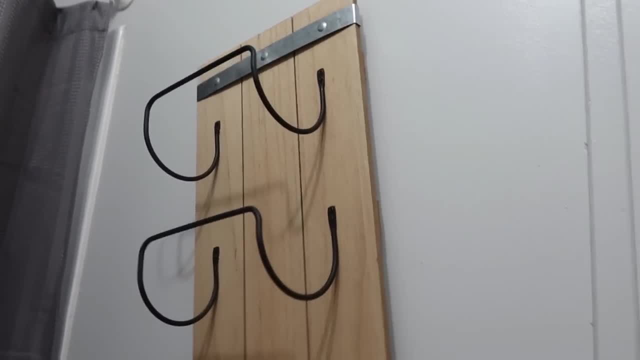 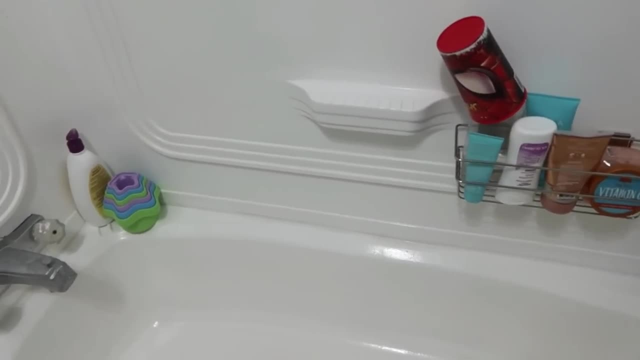 today to where we can use it properly again. I got this from the Dollar General a few months ago and we love it. to store clean towels on. The shower needs some extra storage as well. It's super small and I would like to get everything up off the edges of the tub so that everything. 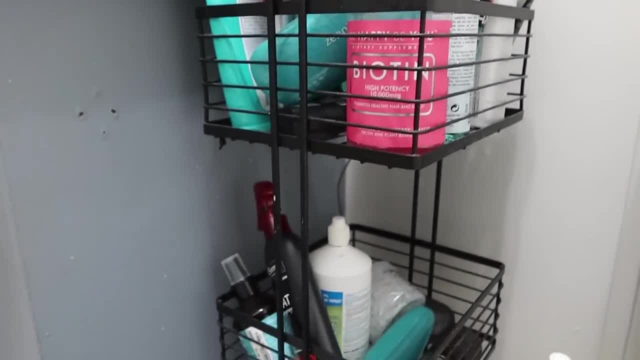 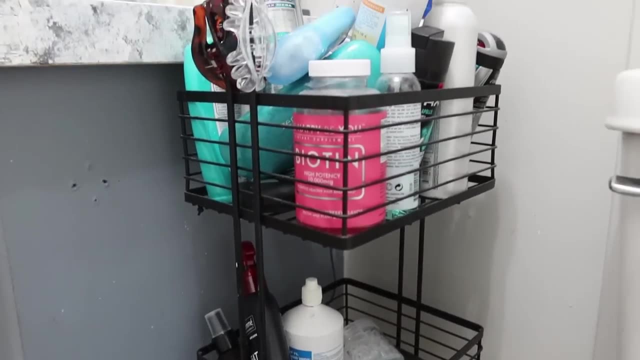 has a place to sit on an actual shelf. I'm also going to be going through all of the products here on this rack and decluttering what we don't use. I get questions about this rack all the time and it's from TJ Maxx. I got it about two or 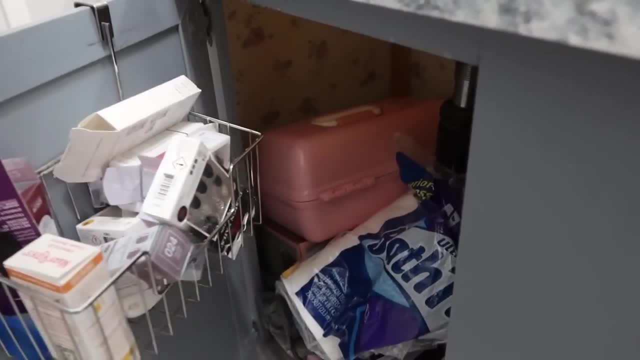 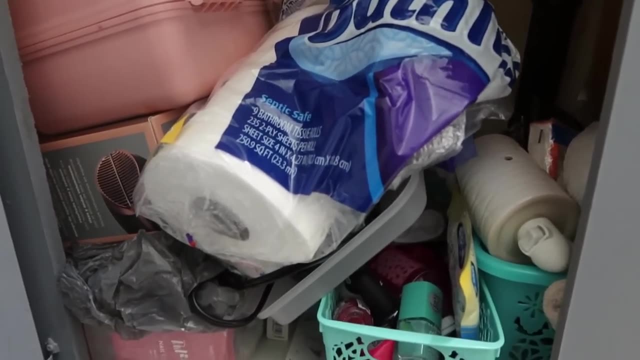 three years ago Under the sink is a complete nightmare. I can't get to anything. I have a lot of things to go through down here, but no worries, The end result is so much better than it is now, so make sure to stay tuned until the end. I'll show you guys all of the 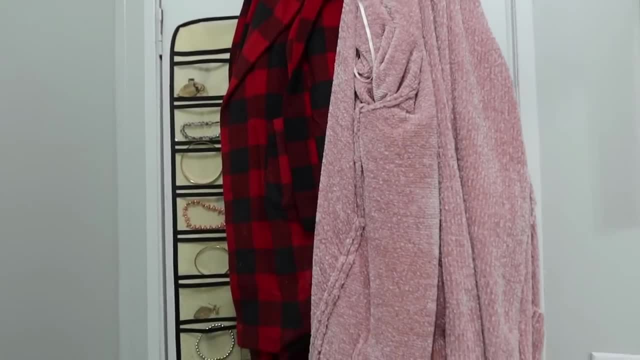 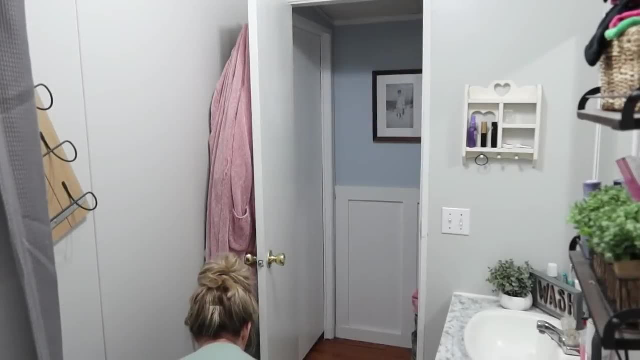 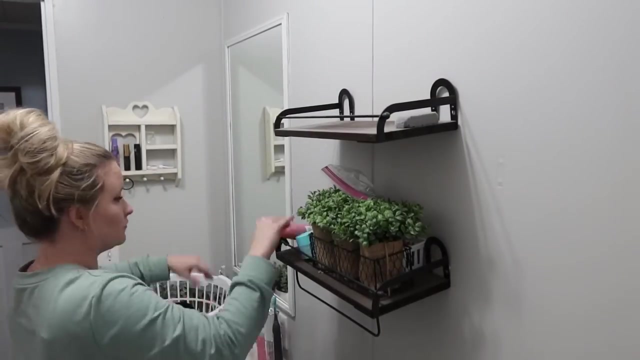 before and afters and also a full tour of how I got everything organized. So the first thing I'm going to do is take the laundry to the washer and get that on and then from there I just started throwing everything into a basket so that I could really go through it, and this way I would have a clean slate when 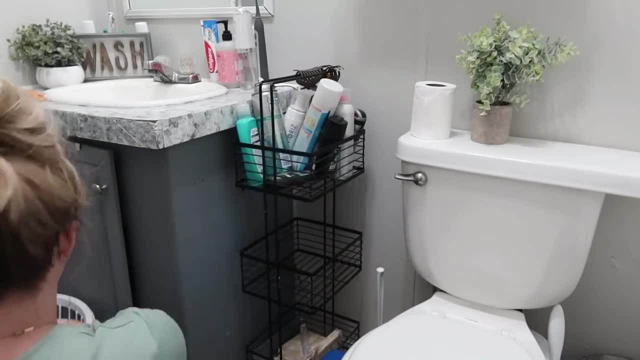 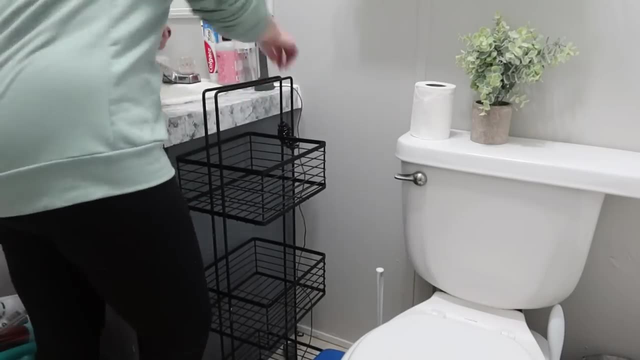 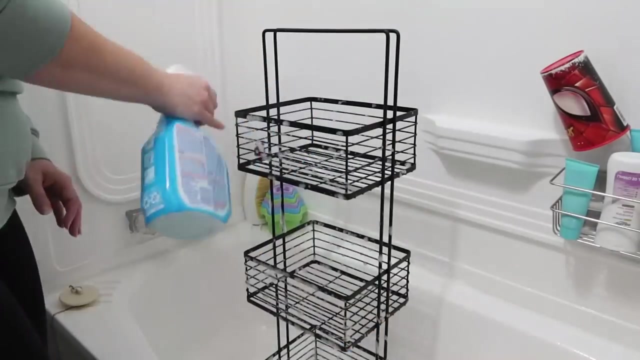 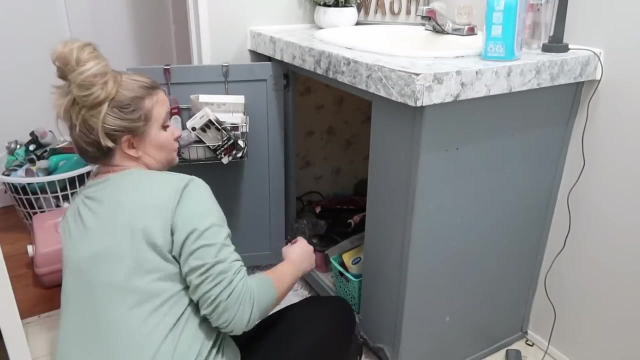 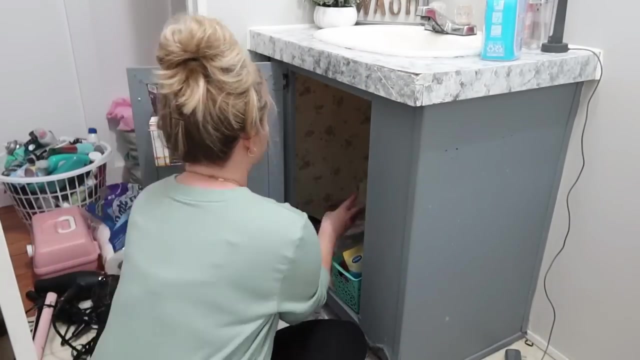 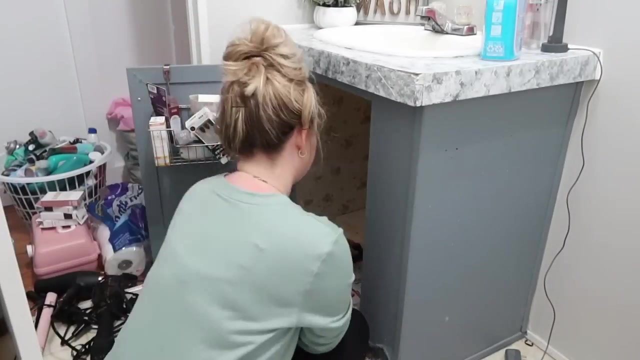 I went to put things back. This rack really needed to be cleaned, so I'm spraying it down with bleach to soak and we'll come back and rinse it off later. There we go. this is my cool little sinkται. So you guys know that I am moving soon and I really want my life to be as 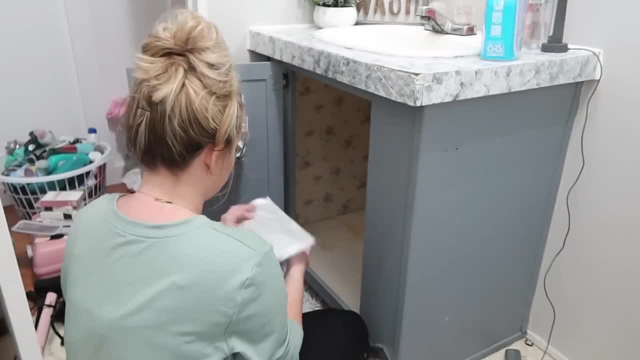 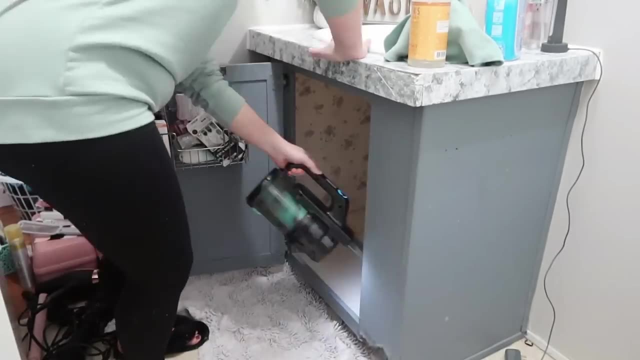 simple as possible when I do go to move. I'm gonna be working on purging things in the coming weeks so that I'm only taking what I need and want, without all of the extra. most of our things are in this bathroom and our bedroom, so I will be 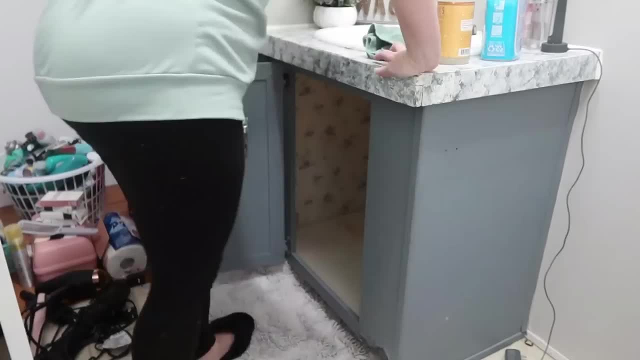 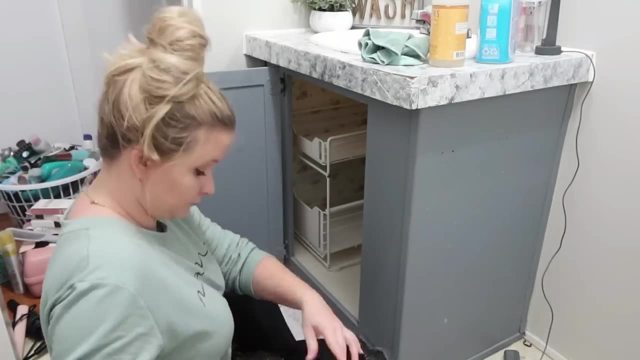 purging my room next, and that'll probably be after the new year before I get to it. but I've got to do a massive declutter before I can start packing, so if you like decluttering videos, make sure to subscribe. I did not realize how. 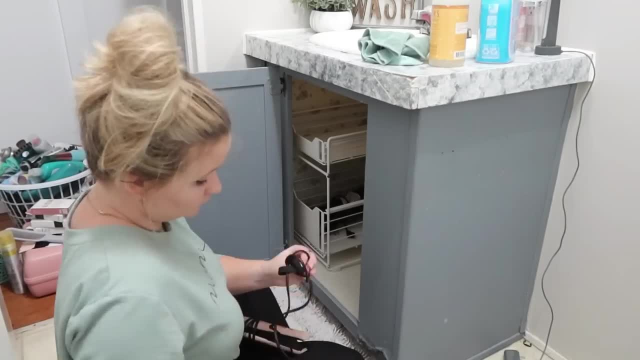 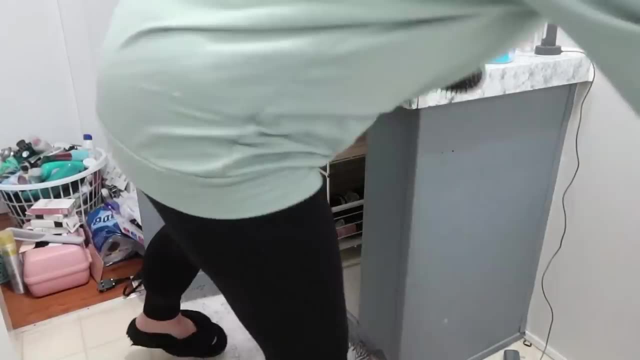 much I had packed into this tiny bathroom until it was all out and on the floor. it was a little bit overwhelming, but it was also the only way that I could actually declutter and go through things properly. I ended up getting rid of so much, though, and I'm really glad that I did it this way. so behind this, 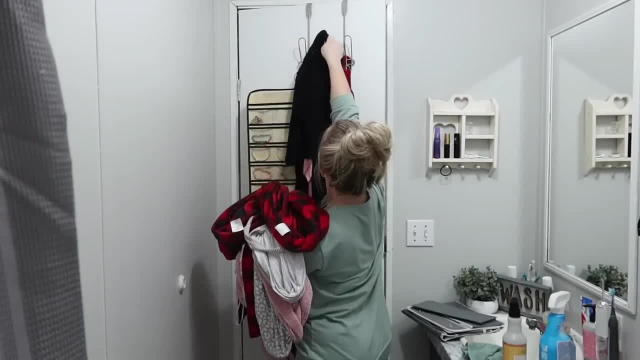 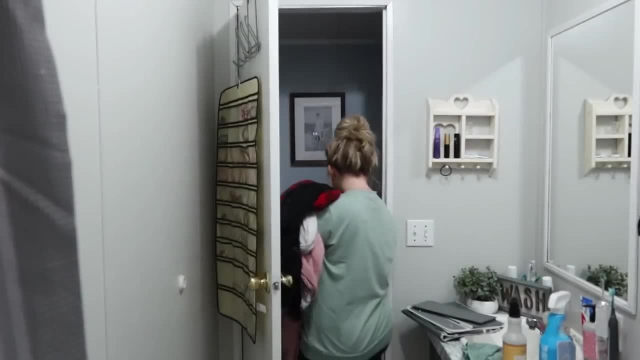 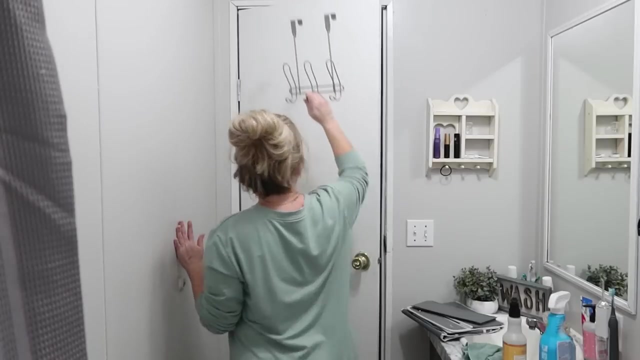 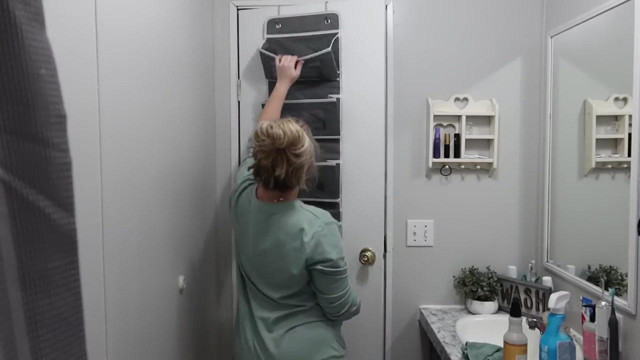 door is where I keep all of my jewelry. it's already organized, so I'll just be moving that somewhere else, and I need to go through my robes as well. I'm going to call you up in the name of love, in the name of love, in the name of love. 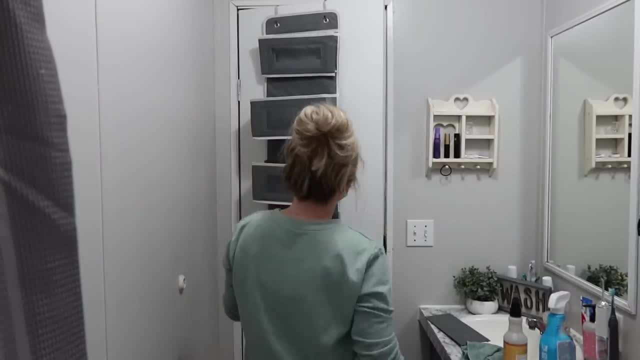 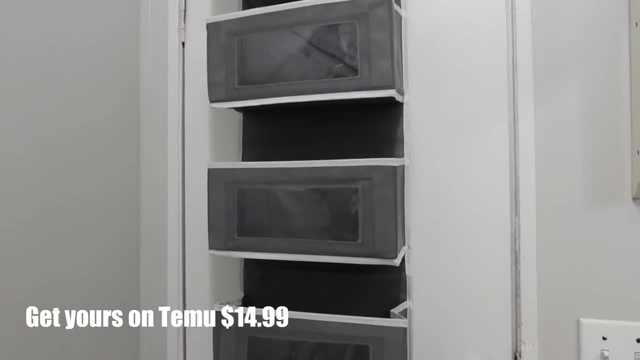 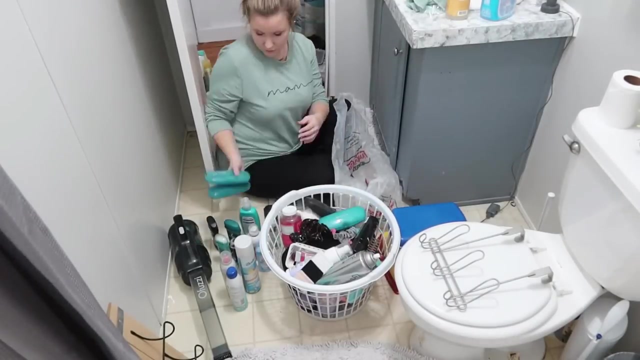 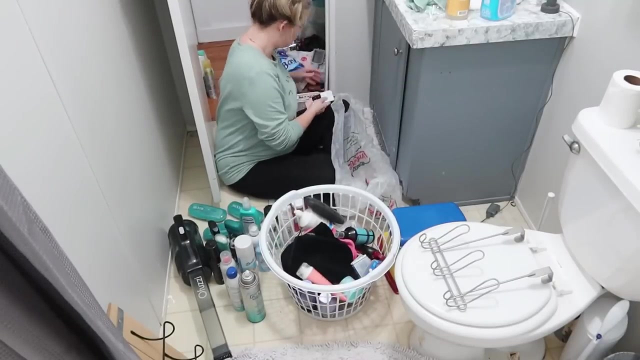 you think you know me, say I'm as cold hearted as they come. you think I'm slowly- no, no, no, cutting my ties with you, that I'm done, but I'm not done. I'm gonna call you up, in the name of love. I'm gonna call you up and tell you that I'm not giving up, in the name of love. 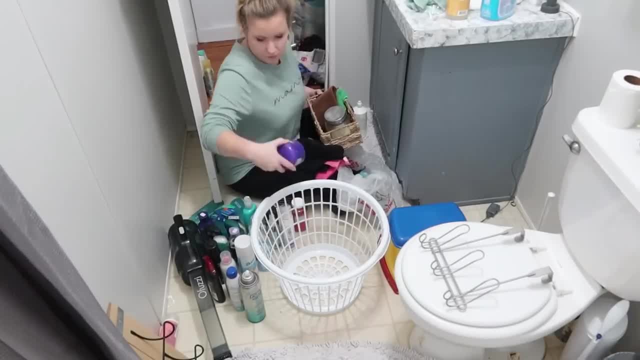 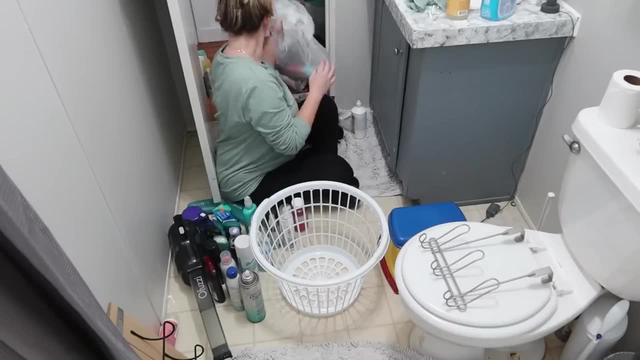 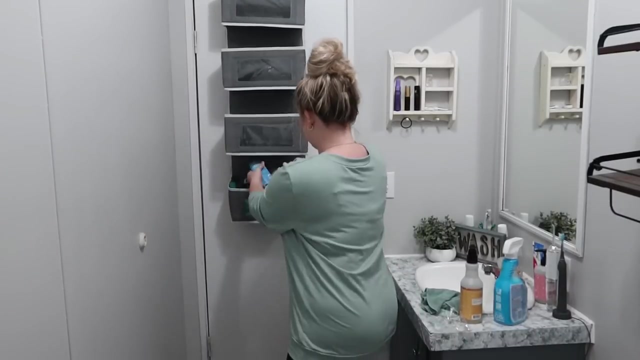 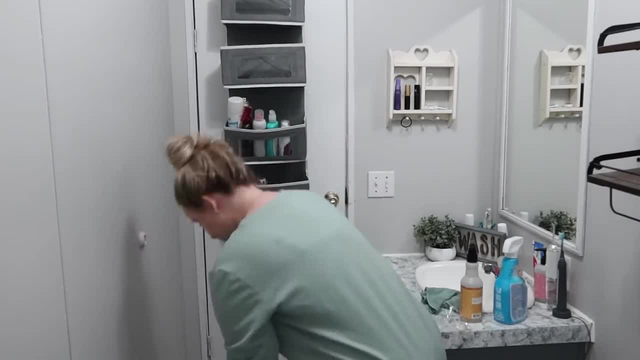 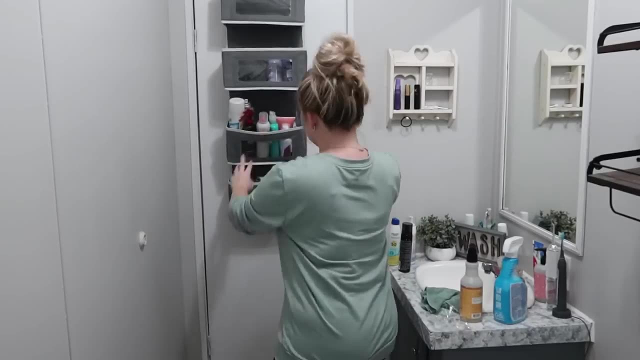 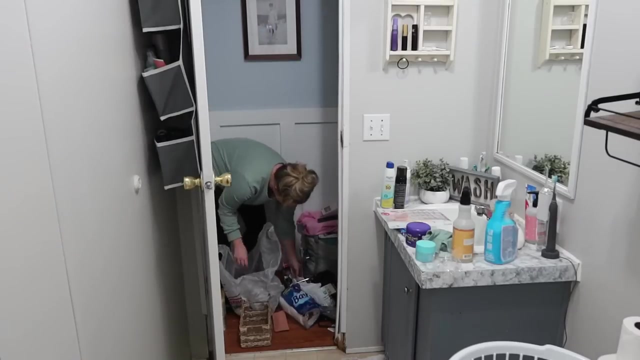 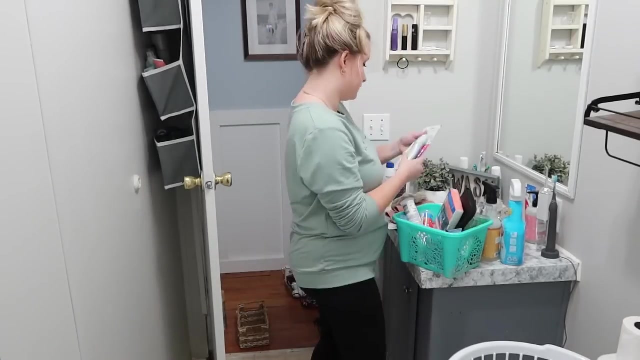 just too heavy and this doesn't do well with heavy items. so I ended up moving those and doing some of my lighter items. I did this- not a lot of dry cleaning out the back of my head. I tried all of my hair products in a day to try to get it out on my other hair. 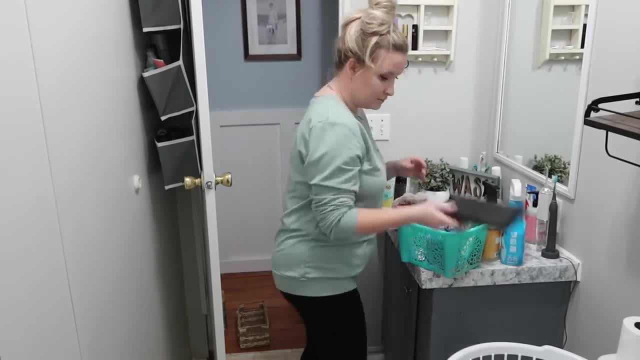 and then I found this mind-blowing makeover, especially of all of it. I didn't know who I was, but it got done, so today I'm gonna give it a try. this is a makeover. it's a look at me with all the hair, and I didn't even know I was wearing a makeover. 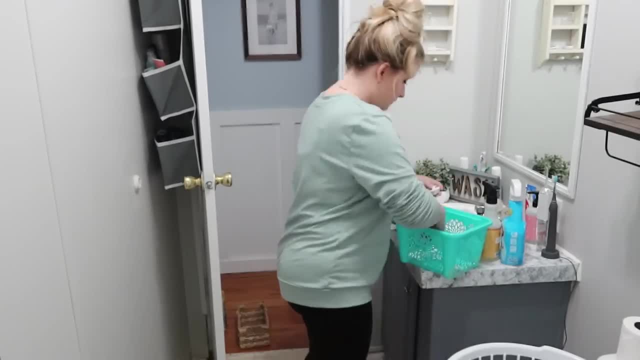 I'm gonna put it on here. this is the edge and this is where I'm gonna start. I'm gonna start and then I'm gonna go for the rest of the hair. I'm gonna go over here. my cuticles are gonna be up there. I'm gonna finish it up. 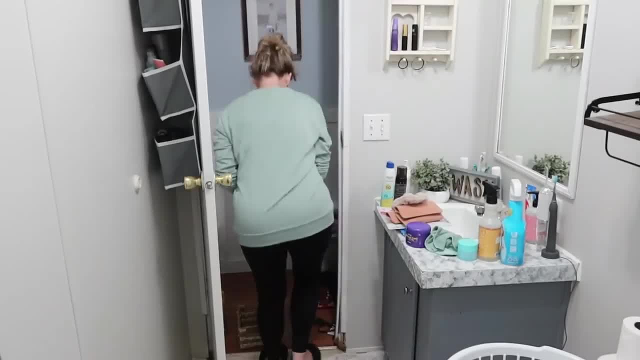 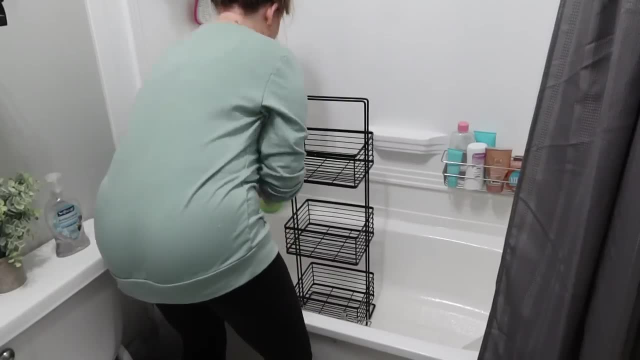 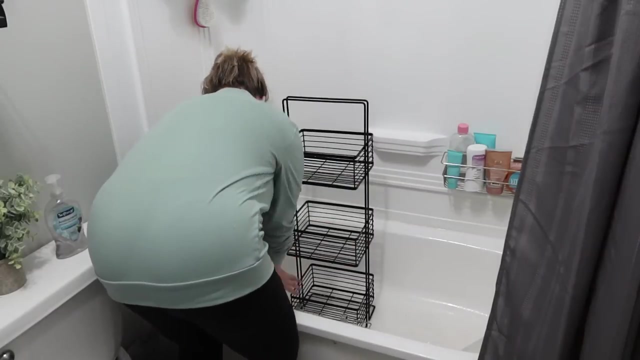 now I'm gonna go back and put my hair in the same place, so let me show you how I do that. when the hair is back- you're new to me, i don't know who you are- be like a piece of art. i want more, but better slow it down inside. my mind is getting all too loud. i get scared. 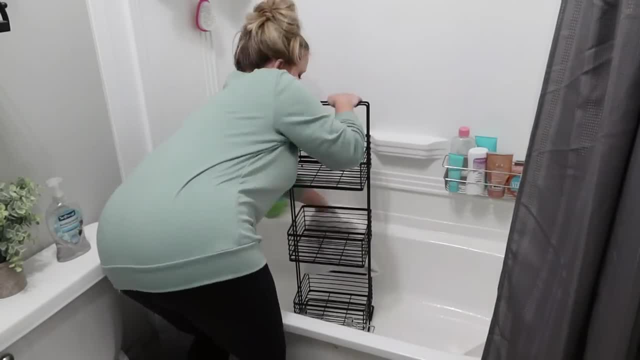 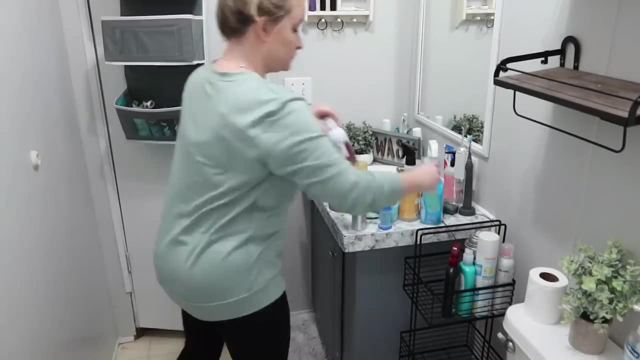 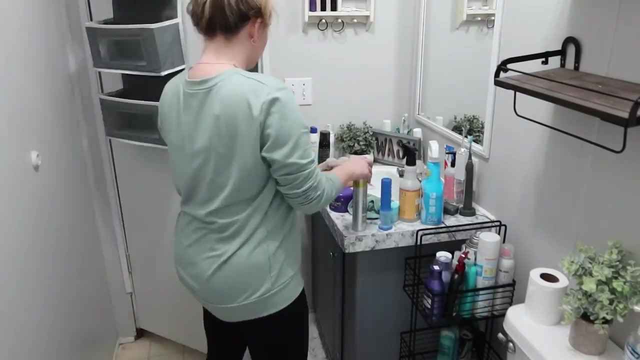 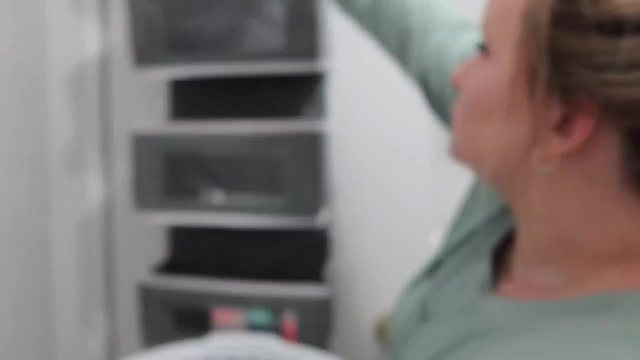 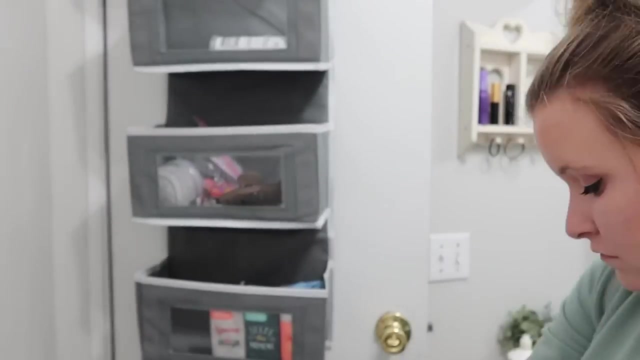 not used to this, not prepared, not used to this. not prepared, not prepared. it was like if we were to waste these moments. they're like poets to me. you are you getting into my brain. i feel emotionally drained. you are you getting into my brain? you getting getting into my brain? 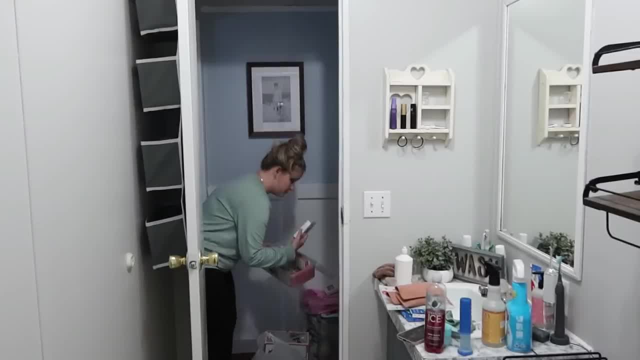 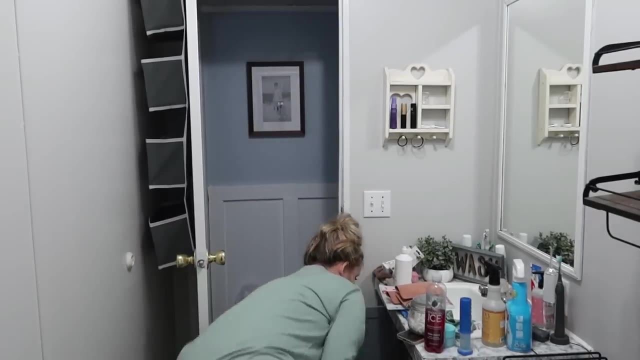 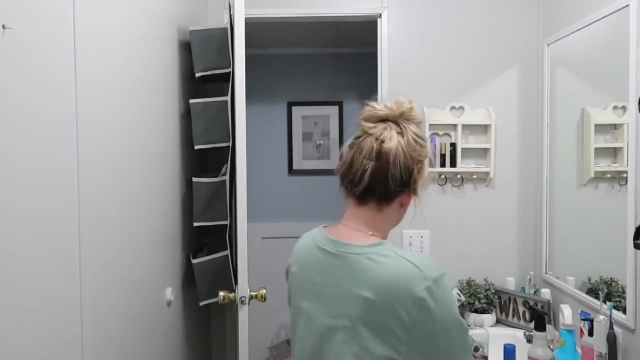 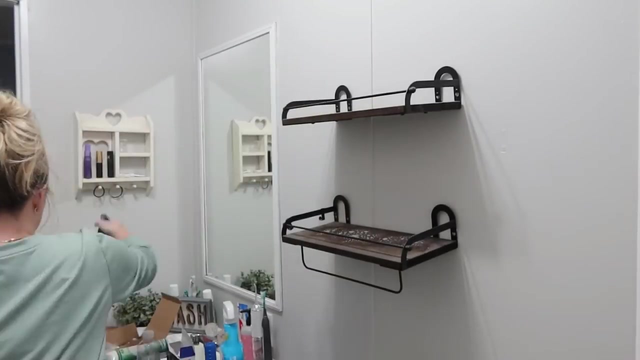 you, you're getting into my brain. you, you're getting this in my brain. you're getting this in my brain. you're getting you getting this in my brain: these shells. you were super dusty, so I'm going to wipe those down really quick and tighten those back up to the 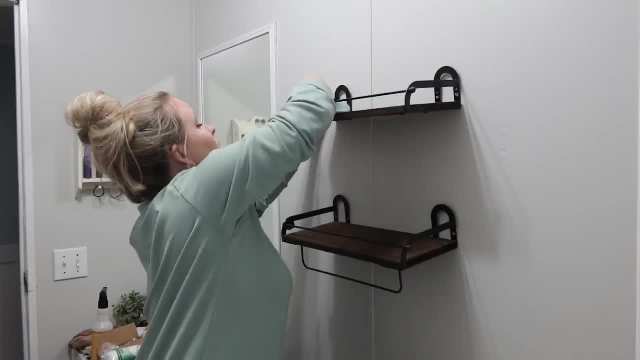 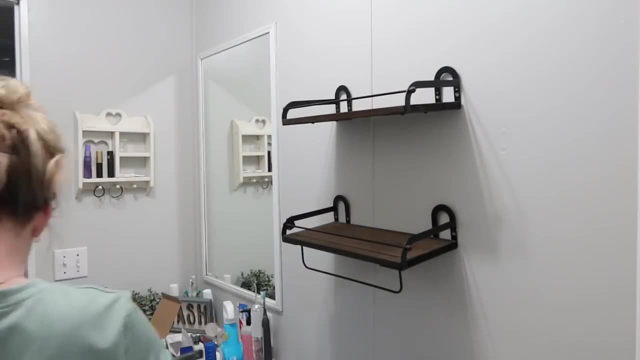 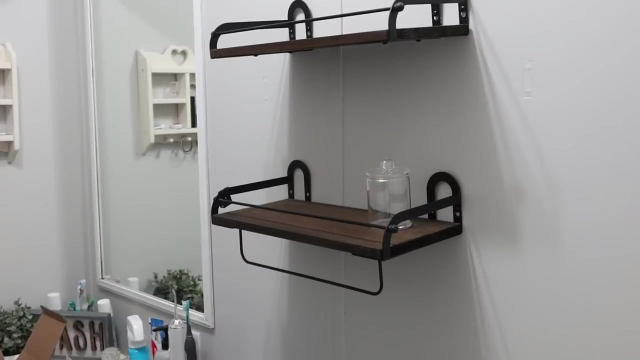 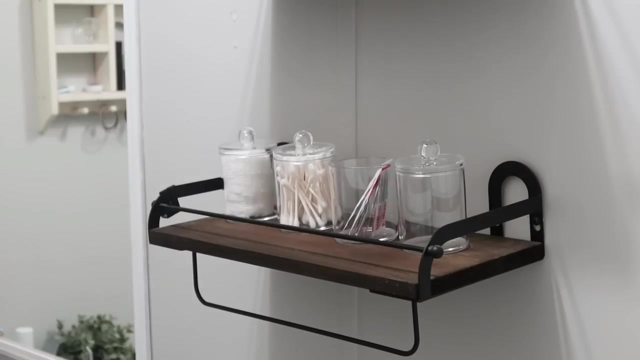 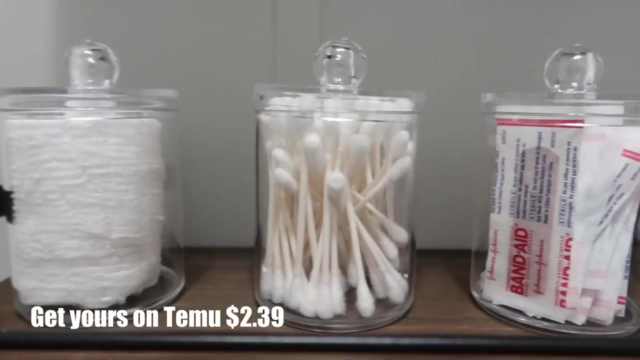 wall. Over time they've started to lean from the weight of all the stuff I had on them, so I just took a couple minutes to tighten those screws back up. you share your love so easily. you share your love so easily. you share your love so easily. 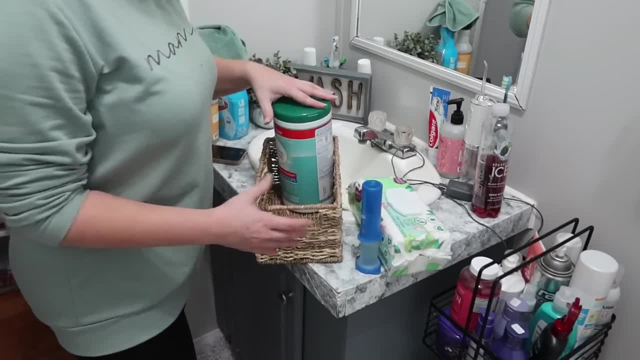 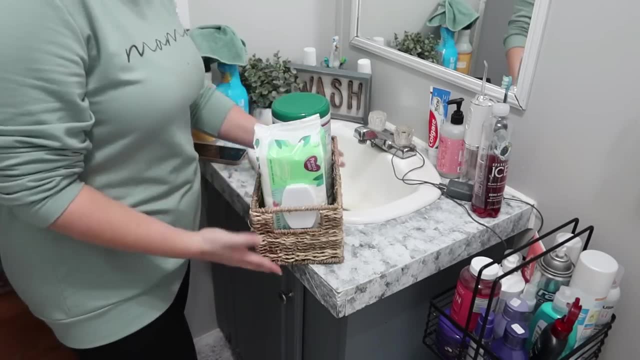 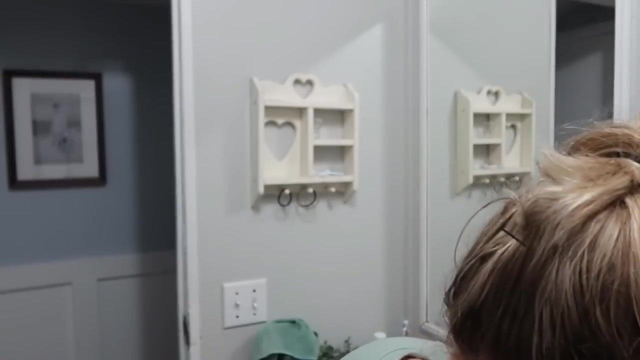 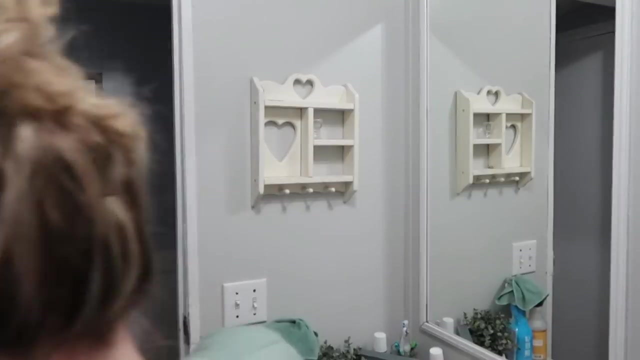 so as cute as this shelf is, it's just not functional. it's really not big enough to hold anything. so I decided just to take it down and hang the kids toothpaste dispenser and rinse cups here in place of it, and I was able to take the 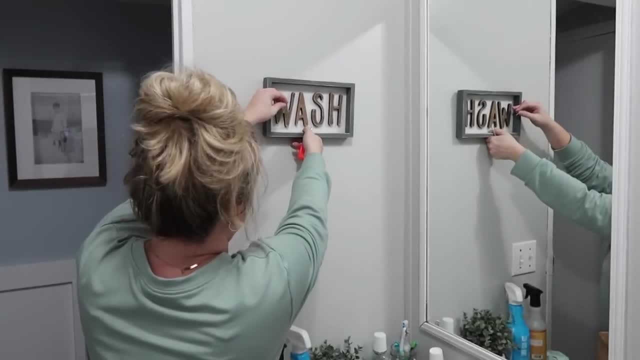 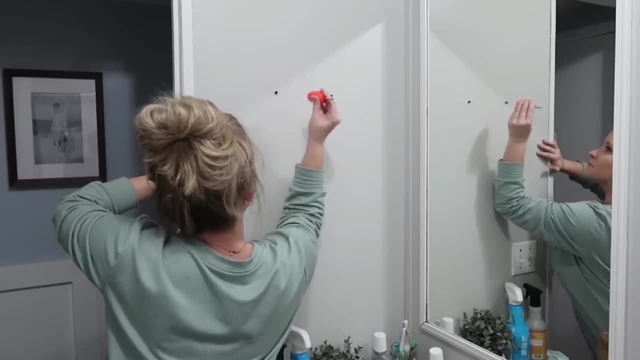 washing machine out of the way and put it back in place, that I had sitting on the counter and hang that up to cover up the screws from where the old shelf hung. I do wish I had the one that said brush instead of wash. it came from Hobby Lobby a few years back and when I bought it there was this: 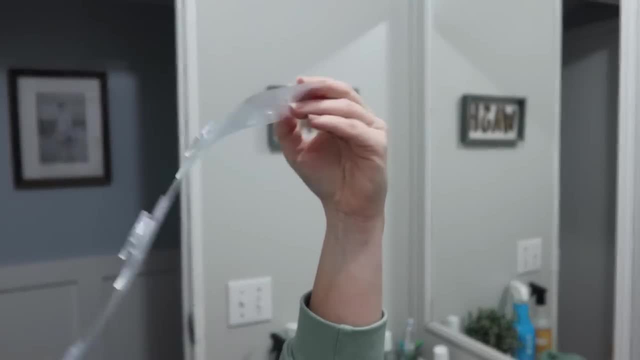 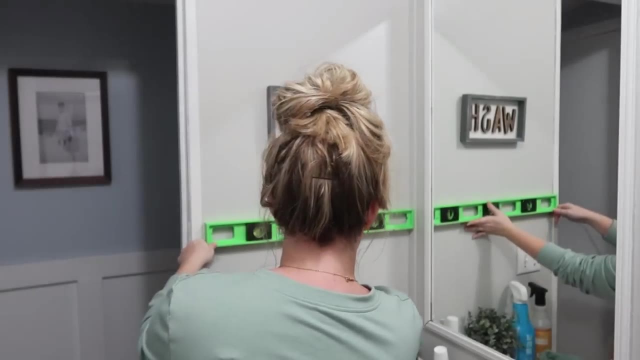 one: one that said brush and then one that said floss. I believe the brush sign would have been perfect, but this is okay too. I love when I can repurpose things I already have and make them work in different places. my favorite thing about these Timu organization products is that they are so easy to use. 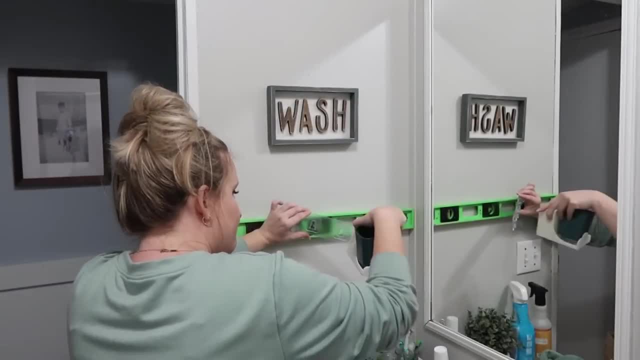 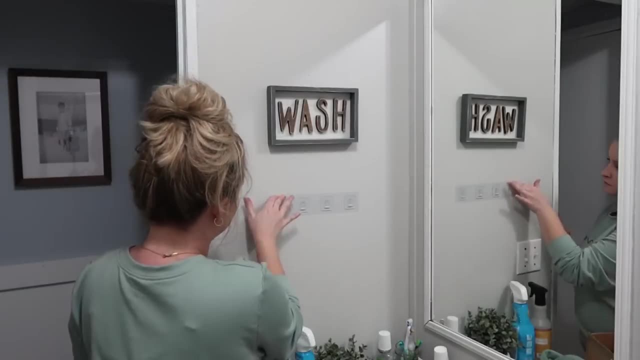 everything is adhesive, so it's peel and stick, super easy to hang. there aren't any nails or screws involved. I don't know how renter friendly it is, though. I don't know if it's gonna remove the paint from the walls when I take them down- if they ever get taken down, so that's something I would have to update. you guys on. I'm saying you care about me, so I do off the call. we're heading down into the dark deep sea gotta dress, but I don't. but here we go again, go again. do my best to pretend, to pretend. yeah, here we go again, go again. 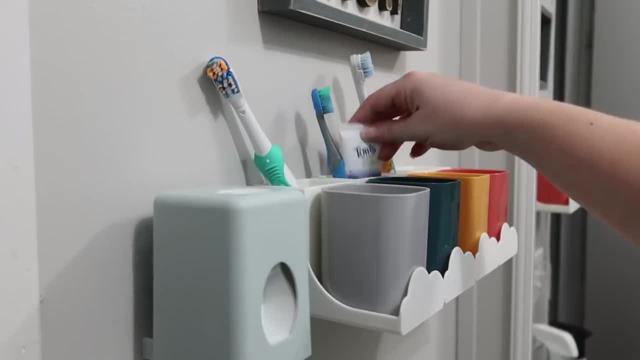 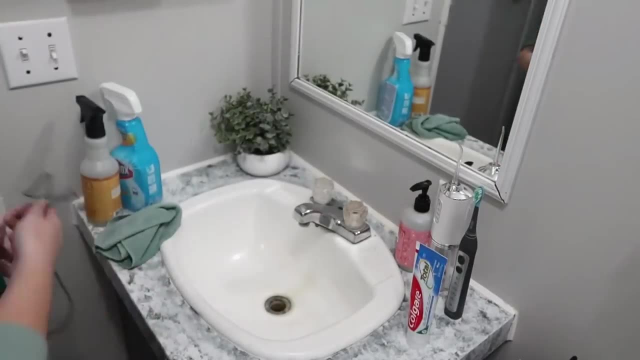 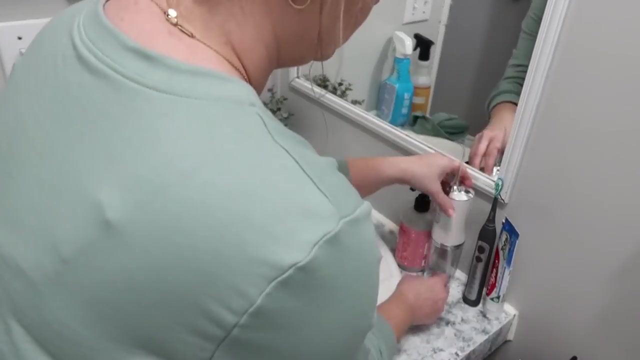 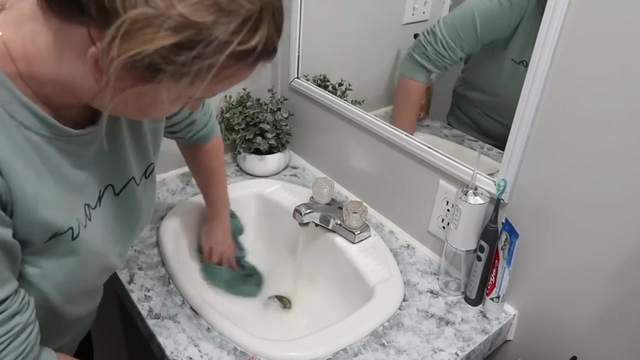 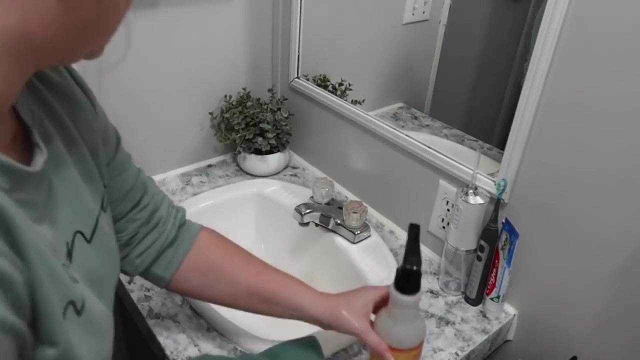 do my best to pretend, to pretend that I don't bother at all, that I'm stronger. but no, I'm in it until midnight. I'm just wondering where you at. just thought I'd call and wish you goodnight. I left my key under the mat. I don't get anything done. you're stuck in my mind. 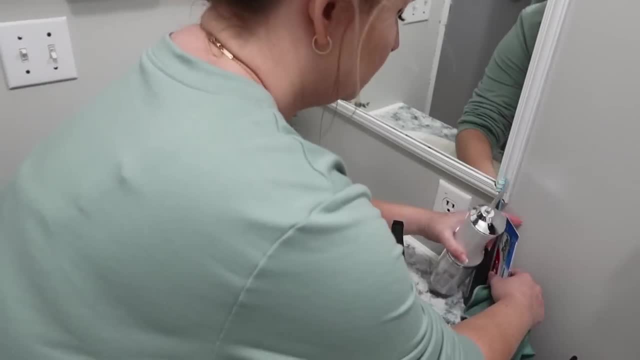 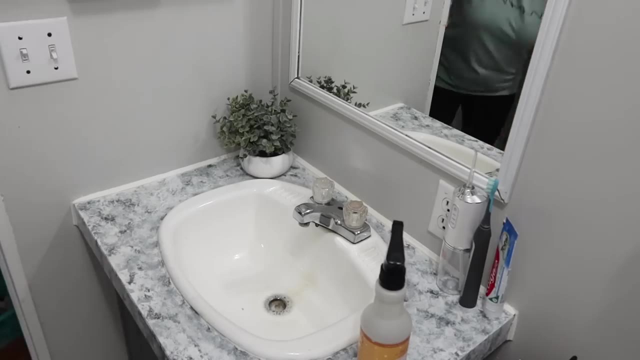 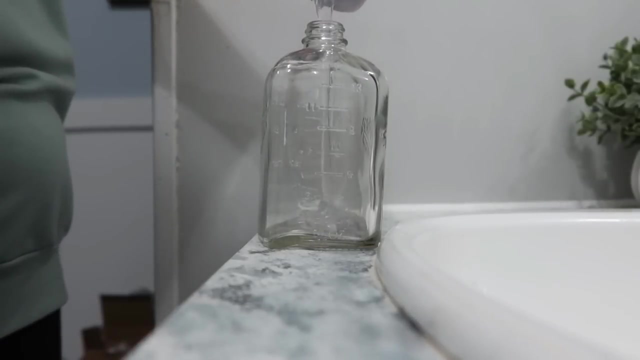 I keep on missing your touch, missing your vibe, this feeling, my girl, when I say we'll be had, won't you come on over, won't you come on over? don't you miss me too. give it all you got babe. give it all you got baby. 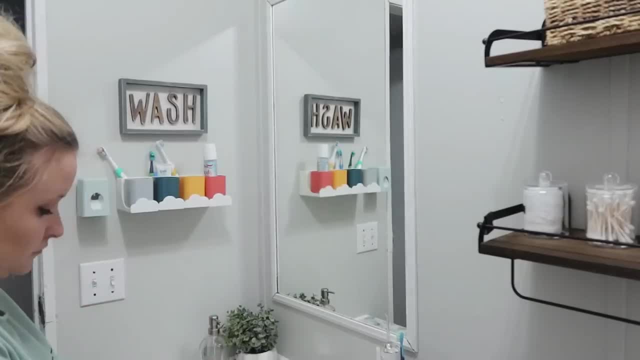 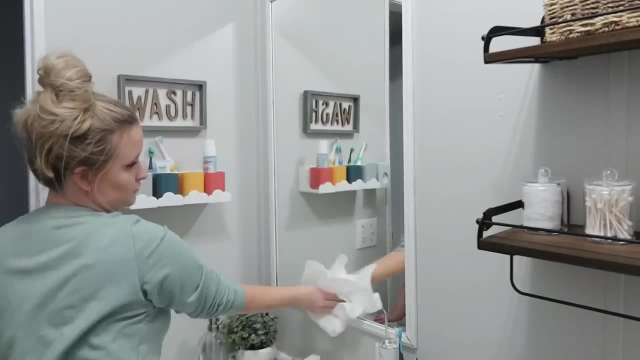 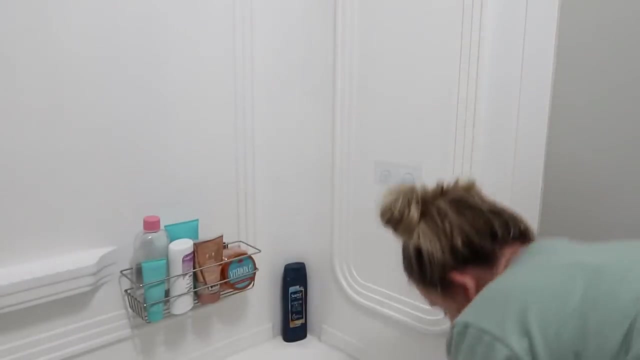 I'd rather try than lose you. give it all you got baby. give me all you got music playing this little shelf. I just ended up placing it on this shelf. I ended up placing it on the shower wall. it came with screws so that you could hang it onto the wall if you wanted. 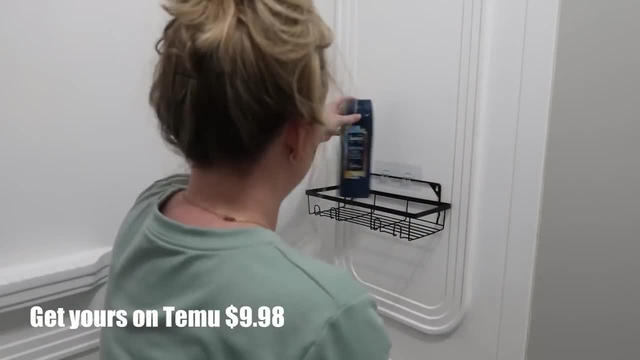 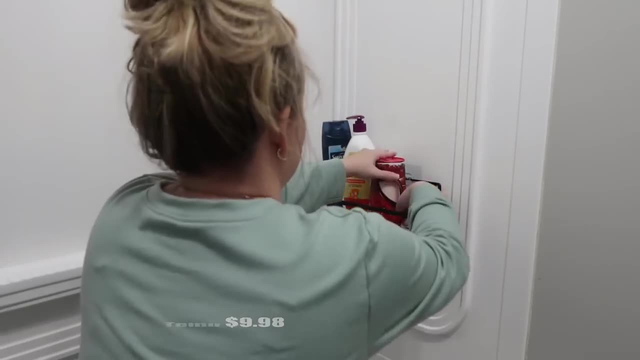 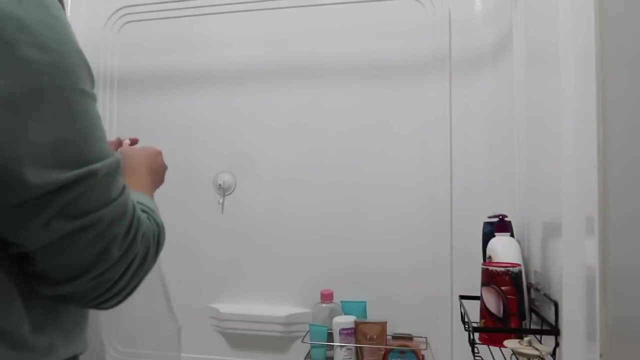 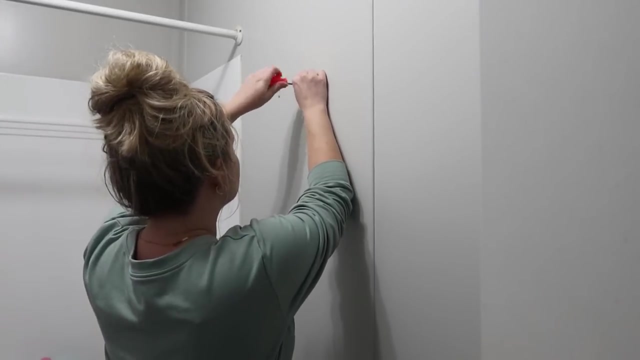 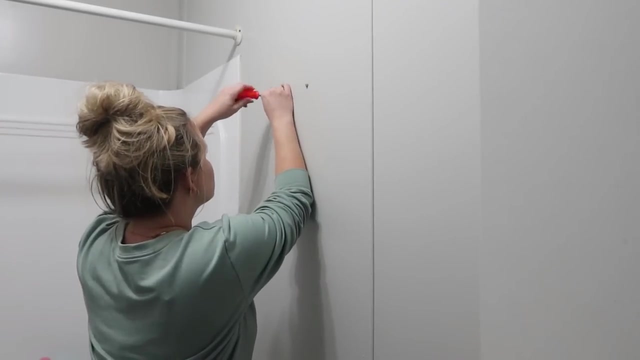 but it also came with the adhesive sticker, so that's what I ended up using so that I could hang it in the shower. music playing: keep dancing in the moonlight. music playing shadows cover up my sins, always murder when in hindsight. but, baby, I don't care to win. 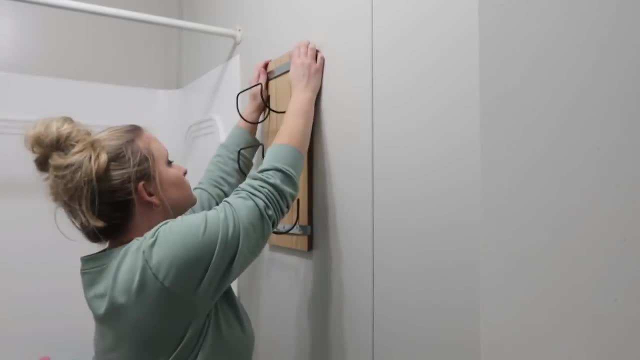 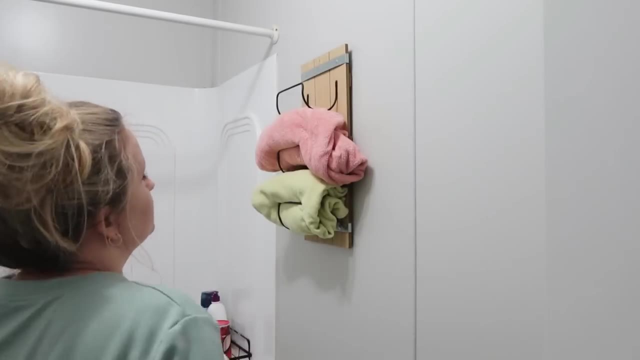 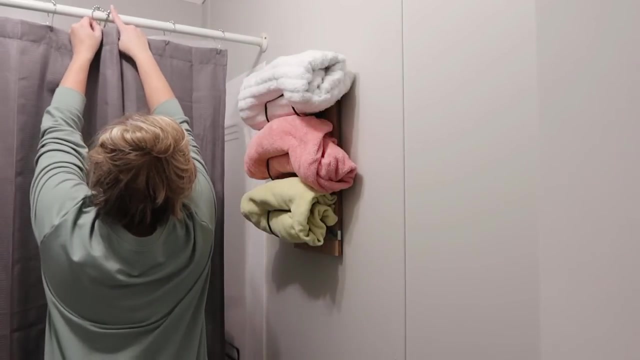 I don't get anything done. you're stuck in my mind. I keep on missing your touch, missing your vibe. this feeling, my girl, when I say we'll be had, won't you come on over? don't you miss me too. give it all you got, babe. 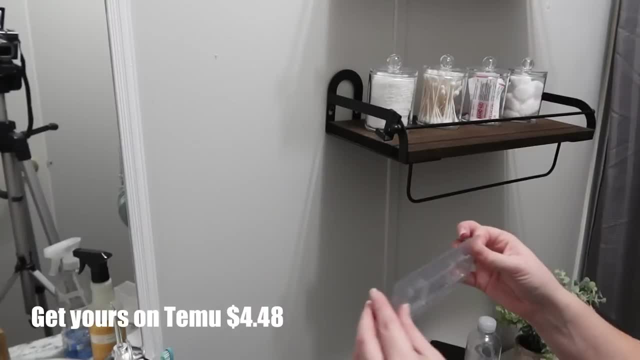 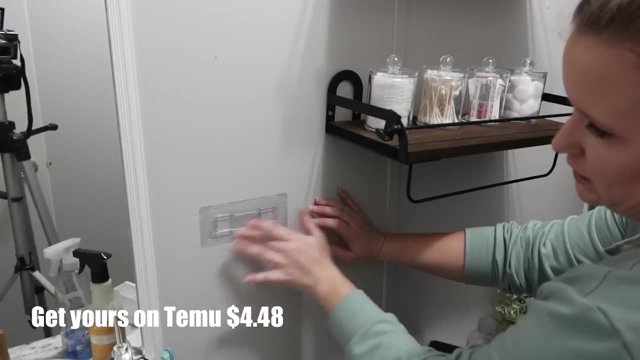 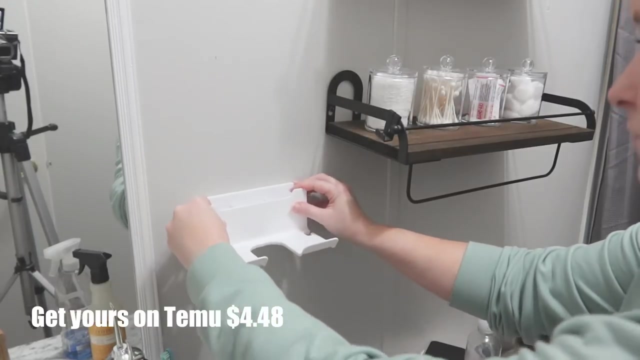 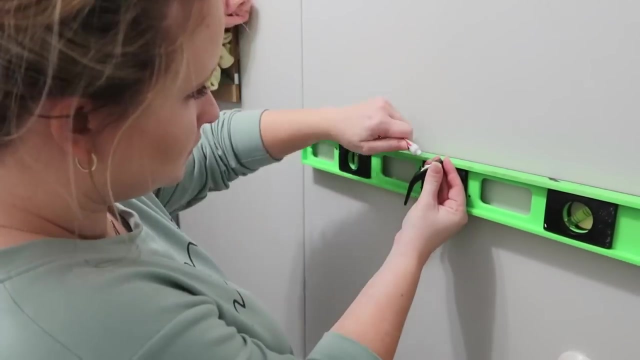 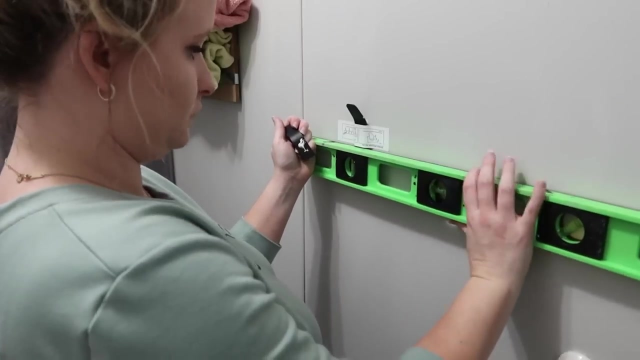 give it all you got, baby. I'd rather try than lose you. give it all you got, baby. give me all you got music playing the towel. hooks are also adhesive. they came with something called MS adhesive that you just squeeze onto the back and then tape them in place for about 24 to 48 hours until they cure. 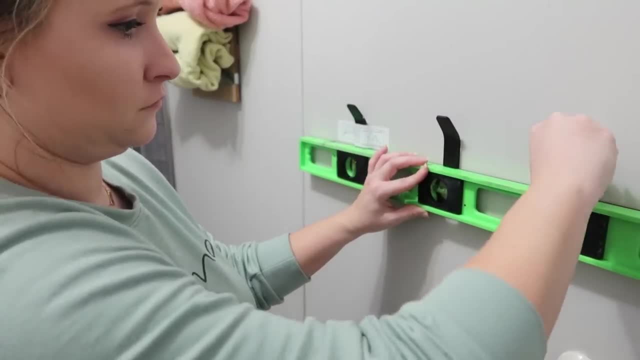 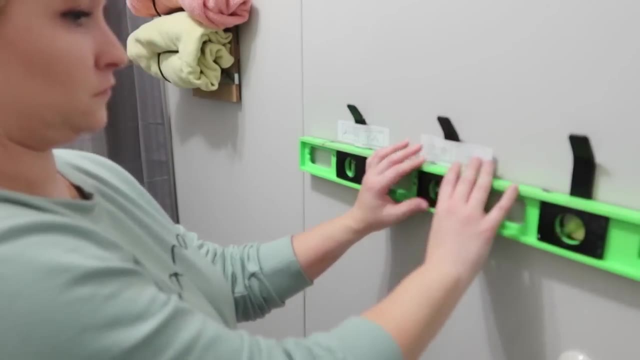 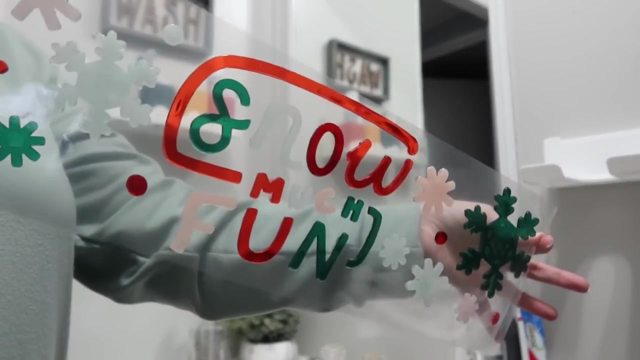 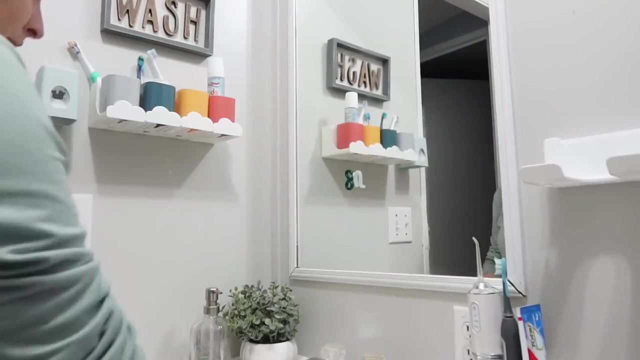 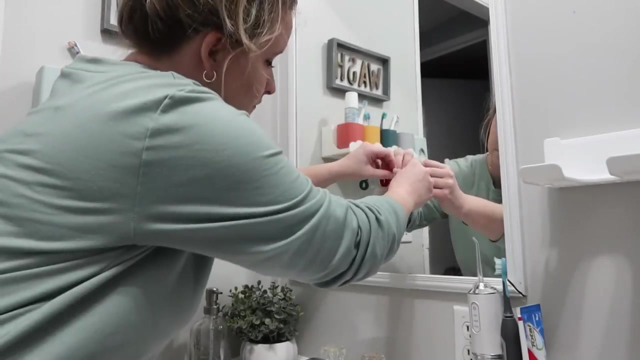 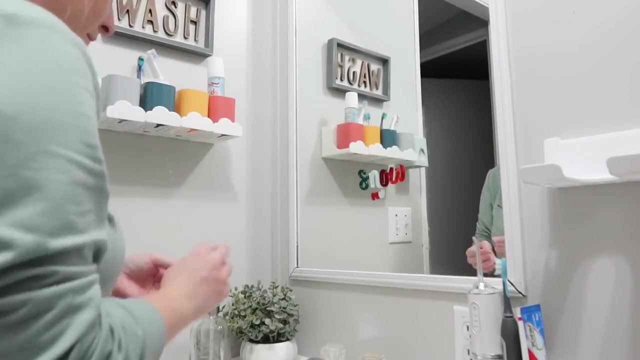 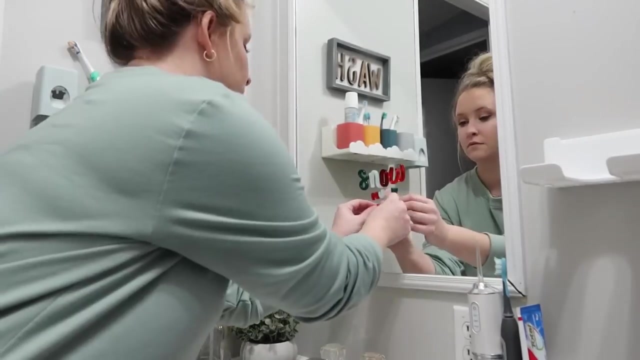 music playing. so for Christmas I thought these window clings from the Dollar Tree would be fun for the kids. it says snow, much fun, music playing, music playing. I don't wanna feel this way, but it's not that easy. you're complicating things for me. no, it's not that easy. 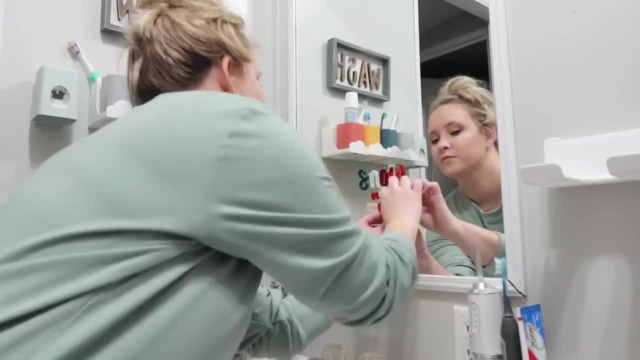 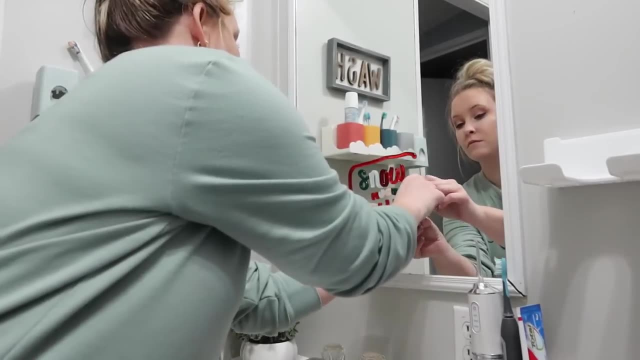 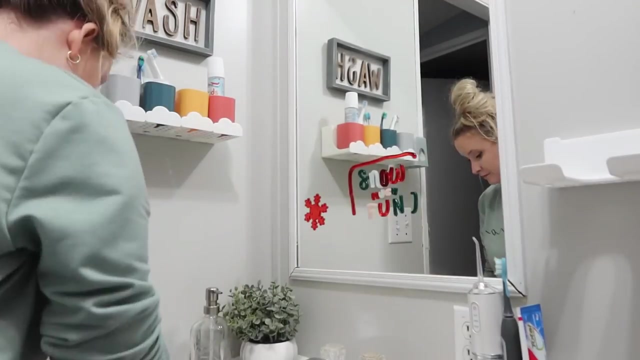 maybe just a little time can heal me, but it doesn't feel the way. what are you doing to me? music playing. why'd you break my heart? music playing left me in the dark, dark music playing. why'd you have to go music playing? I don't wanna feel this way. 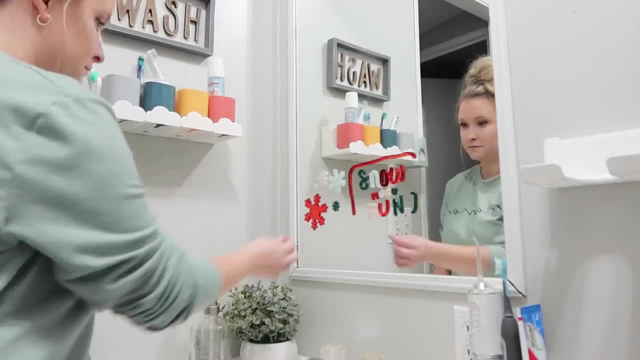 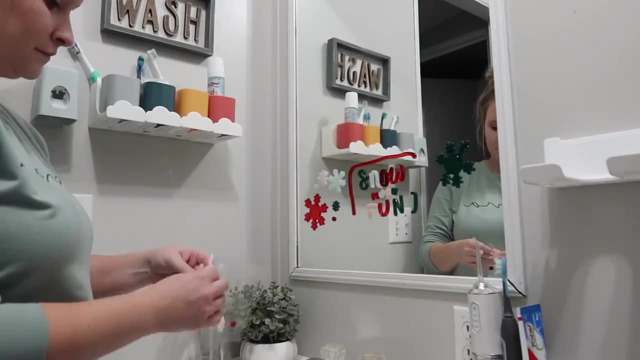 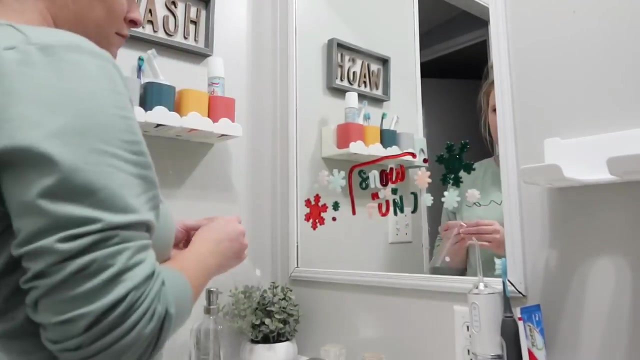 music playing. though I'm broken, I'm still hoping I could be with you music playing. I'm still breathing. it's not easy. I'm just a. I'm just a hooo, hooo, hooo for you music playing. one last thing I'm gonna do is give the floor a vacuum. 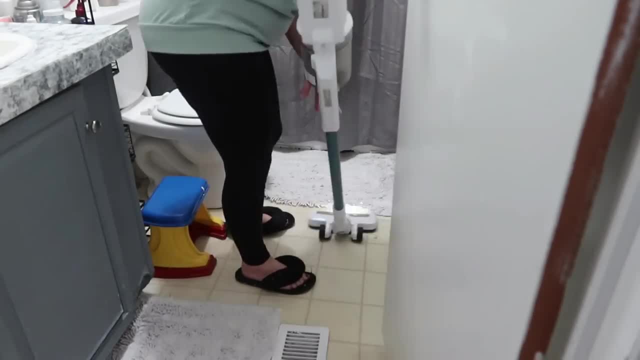 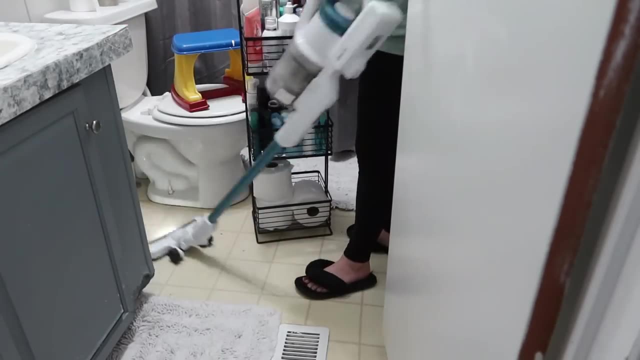 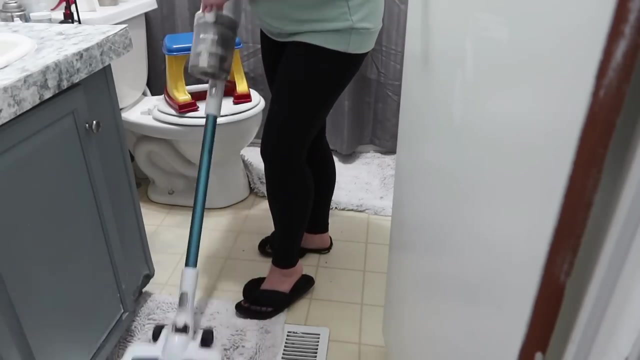 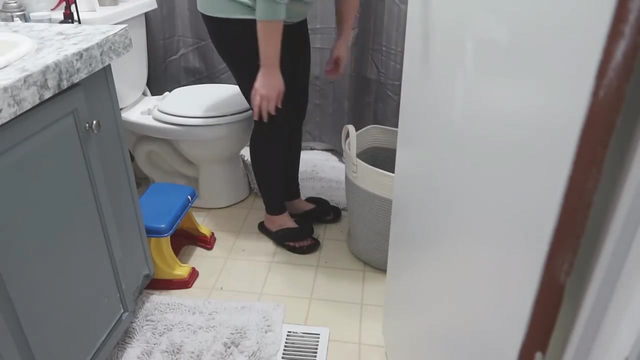 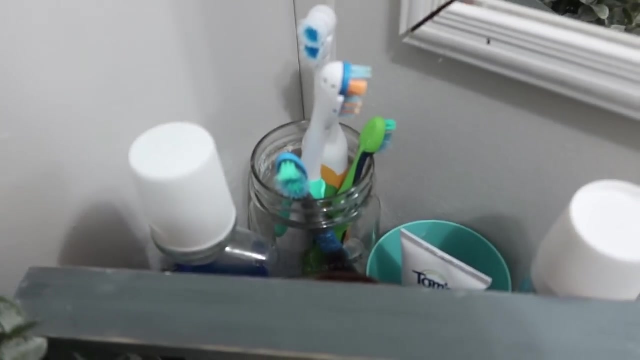 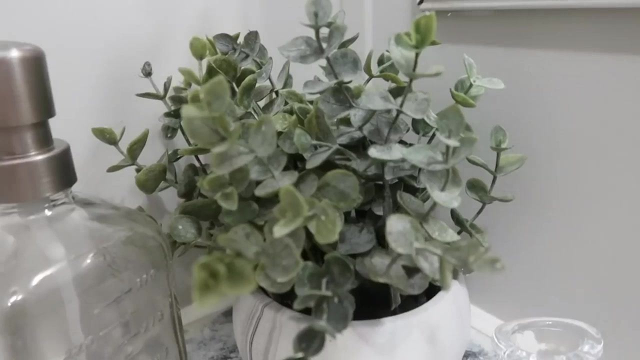 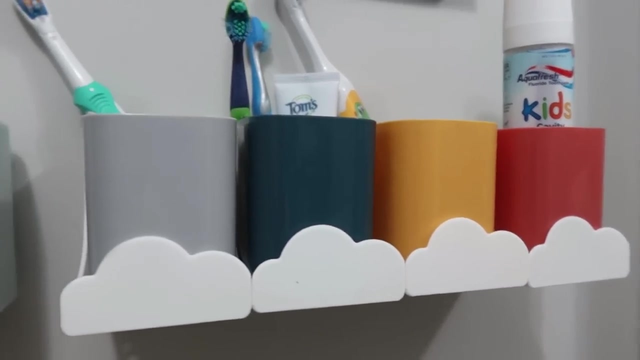 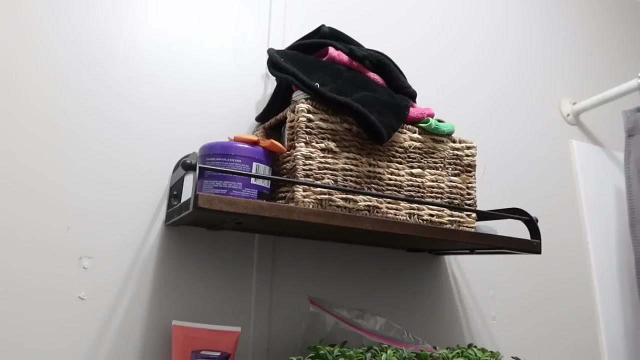 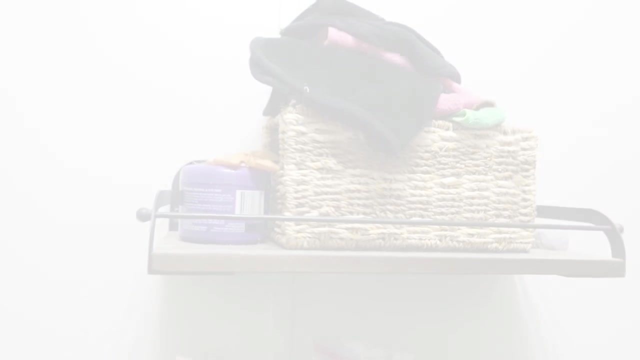 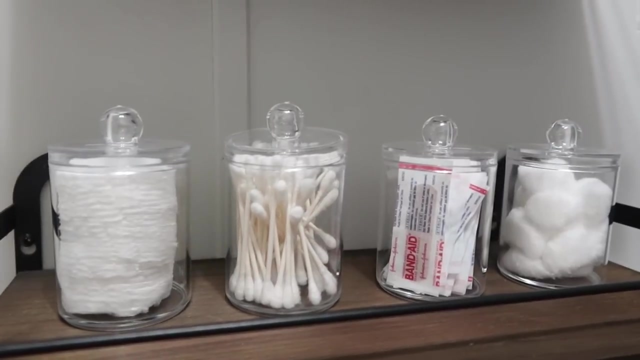 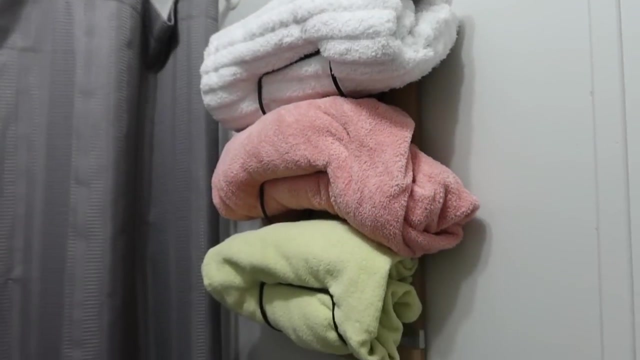 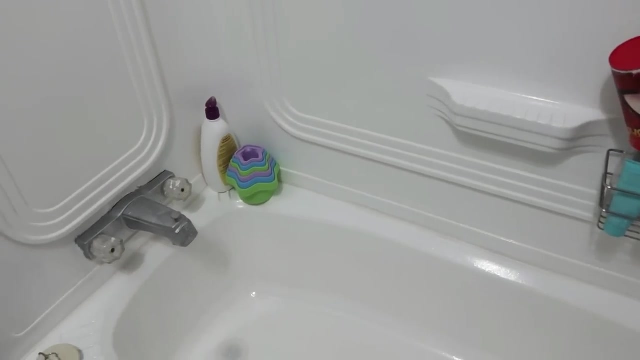 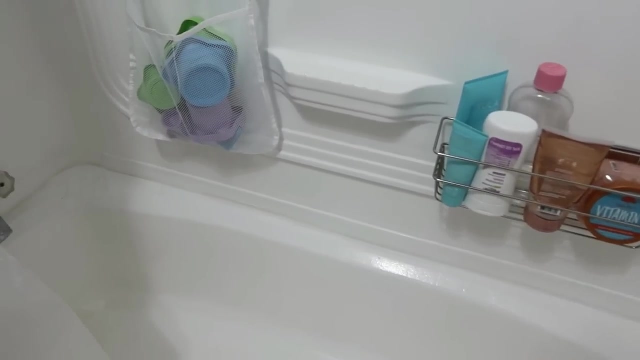 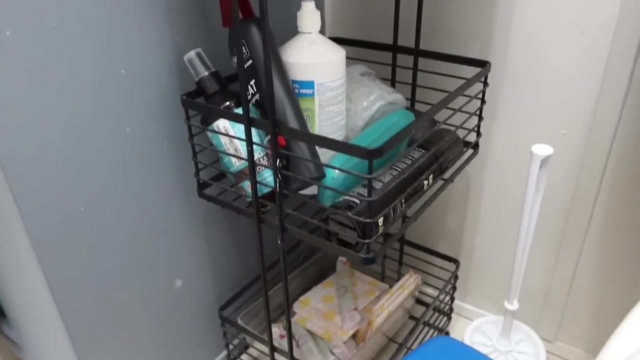 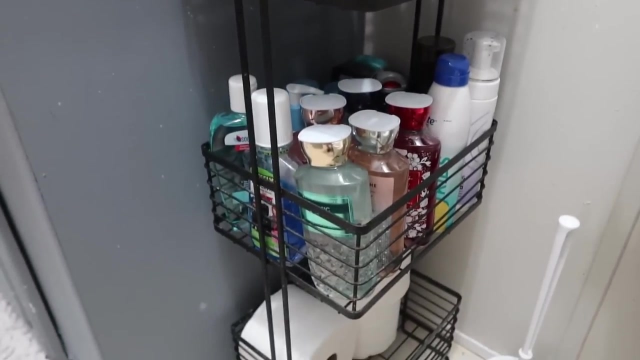 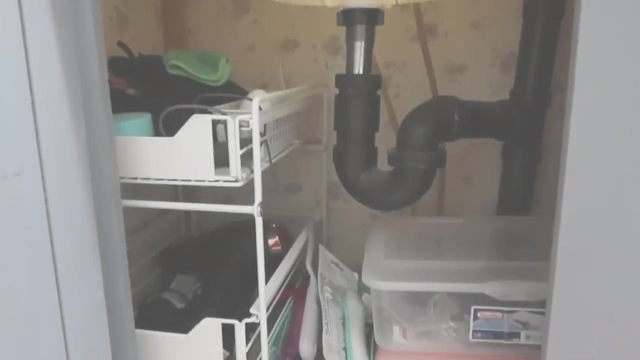 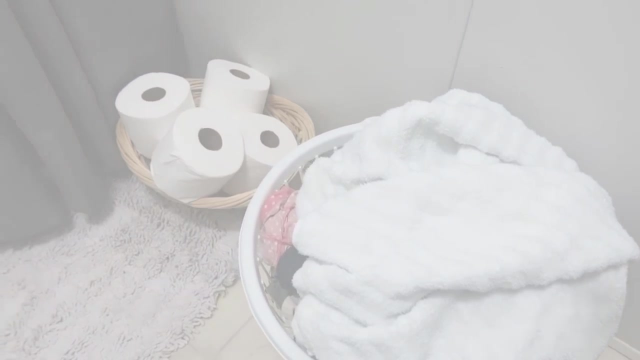 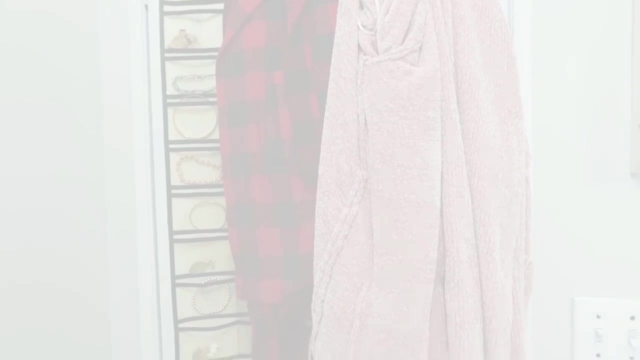 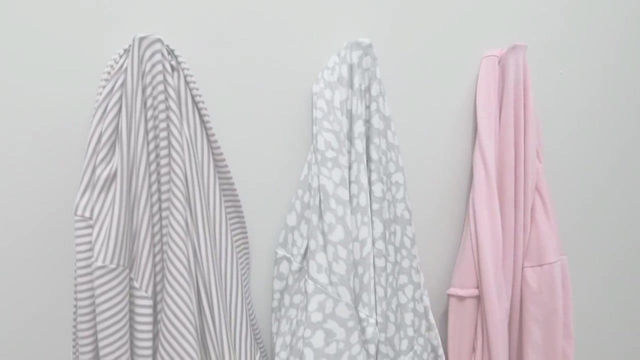 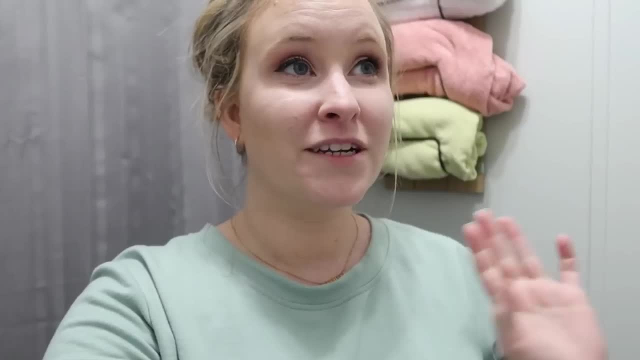 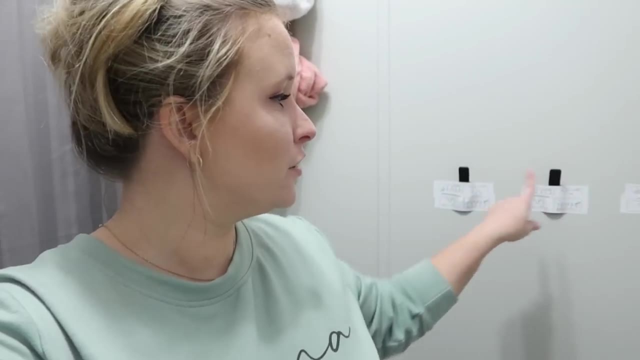 It looks ten times better than it did. So I'm going to show you guys a tour of kind of how I organized everything. I do still have to wait on my towel hooks to cure. You can't take the tape off for like 24 to 48 hours. 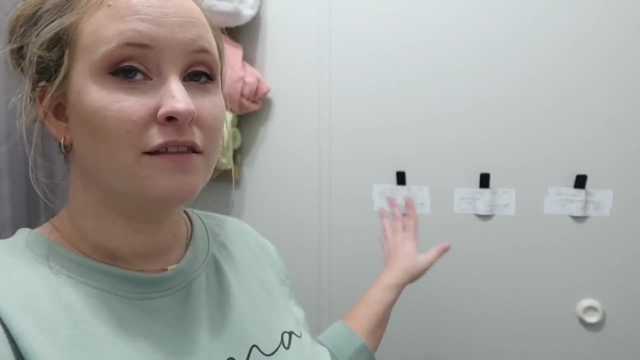 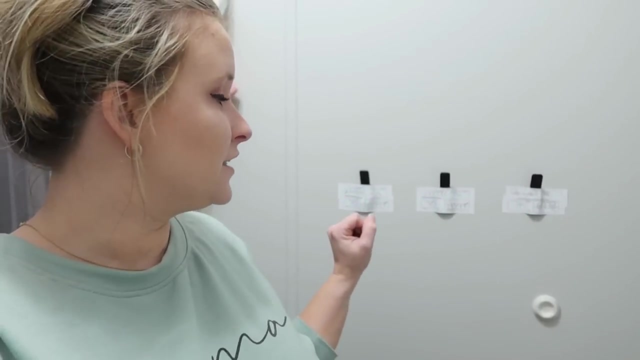 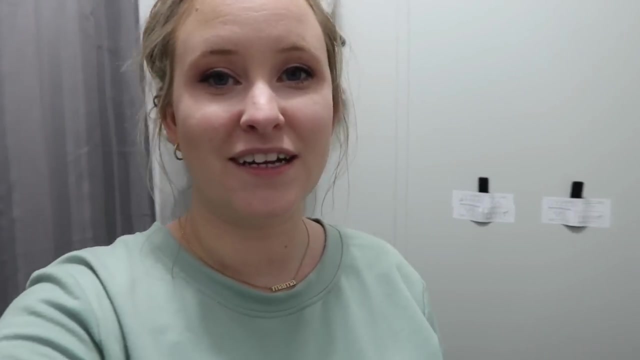 So I'll check them tomorrow, see where we're at and then go from there, But my plan for these are to hang my robes on those instead of actually using them for towels, Because we have this there. But anyways, let me go and flip you guys around and I'll show you guys a tour. 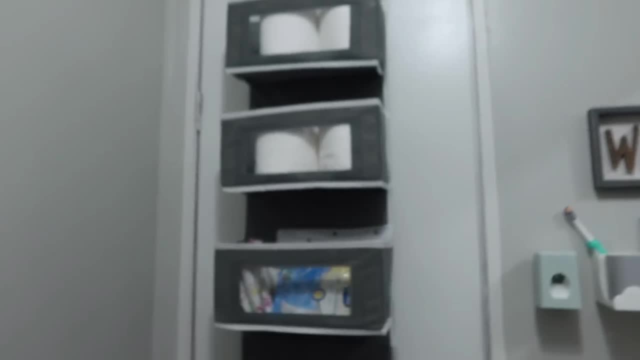 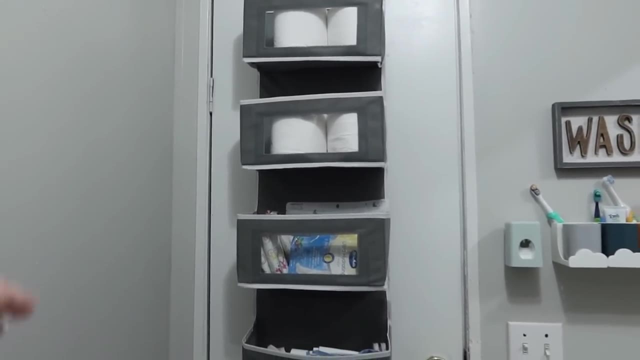 Okay, so let's start with this over-the-door organizer. This was literally so perfect. Like I said in the beginning, this would be great for a baby's nursery. You could put diapers, wipes- all those little gadgets that newborns need when they're first born. 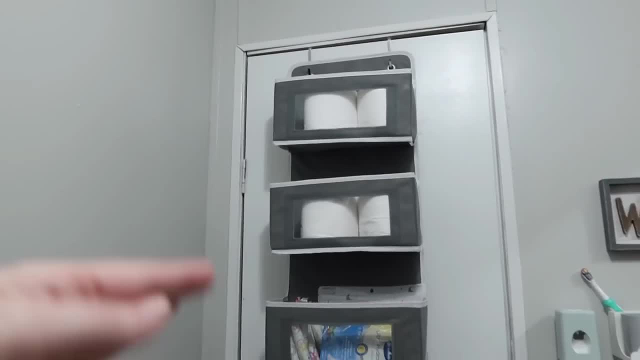 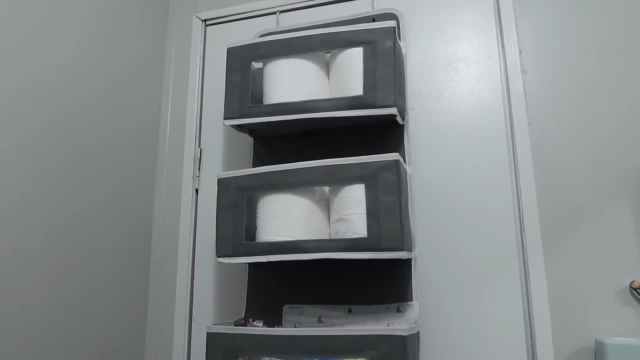 It would be so perfect for a nursery, But, as you can see, it's also great for a bathroom. So up top I have some extra toilet paper, So I was able to get our toilet paper up off the floor. We literally had nowhere to put toilet paper. 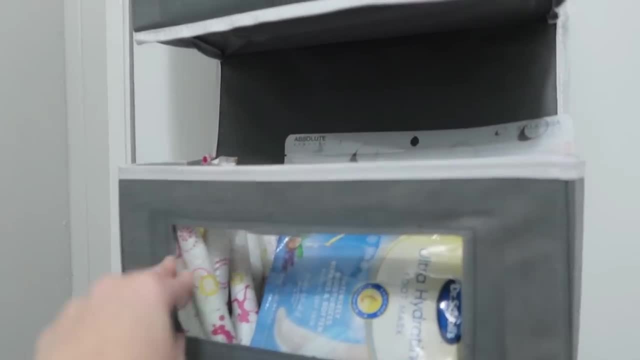 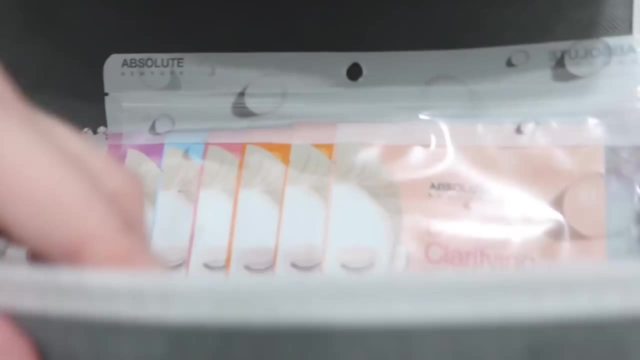 So that fixed that. I've got some extra feminine products. This is like miscellaneous stuff, by the way, too. I don't have it like perfectly organized, But I've got a foot mask, a thing of like face mask in there. 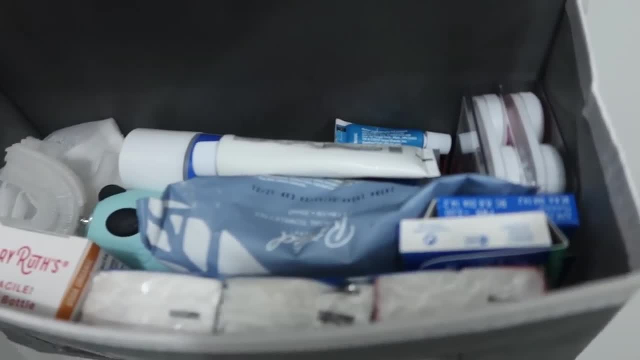 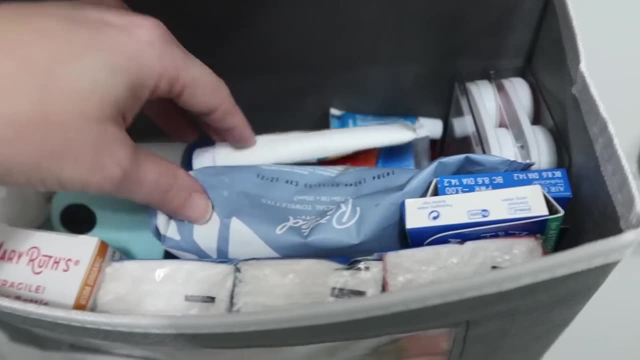 And then this one on the bottom has like extra toothpaste, Some of the kids', extra little toothbrushes that actually need to be charged, Some Kleenexes, extra contact cases, just little miscellaneous things like that. Um so, 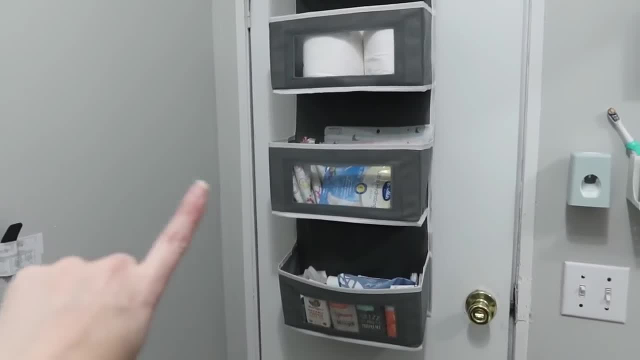 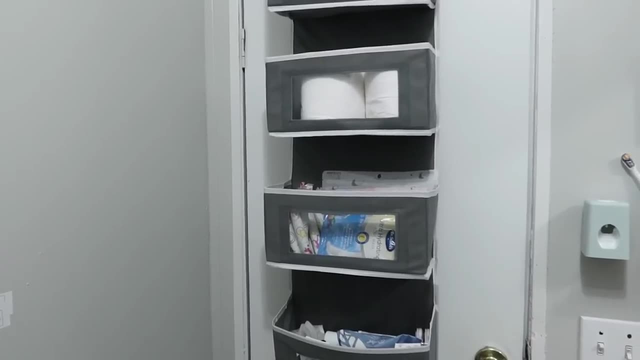 Makeup remover wipes my contacts. This is much more functional than my jewelry organizer that I had here on the back of the door, So I'm gonna do something different with my jewelry. This gave us a lot more storage space, So I love that. 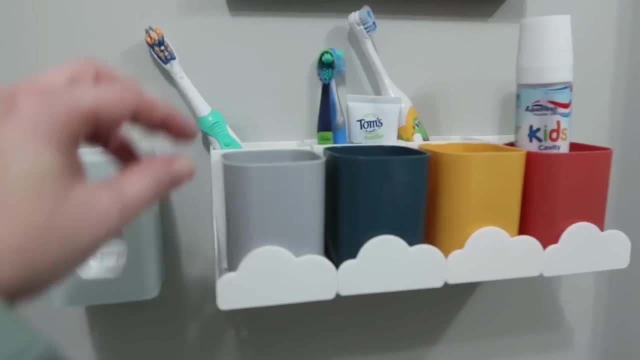 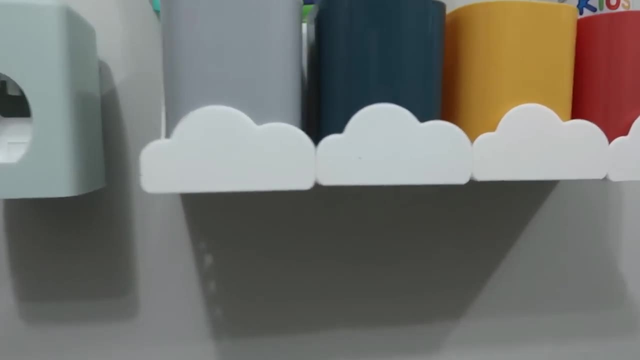 This is actually my favorite thing in the whole bathroom. It's so cute. I like how the cups are different colors, So everybody has their own color, and the toothbrushes are actually supposed to be able to go into the bottom, Like the heads of them are supposed to slip up through the back, right there. 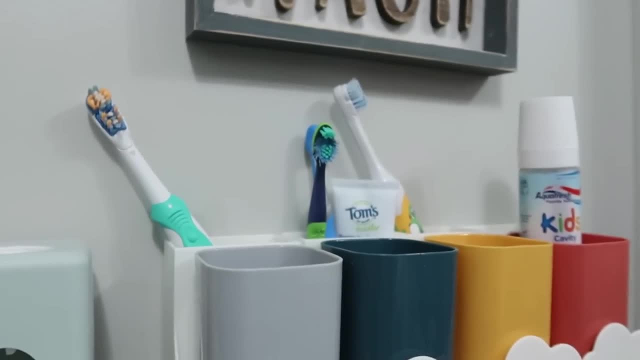 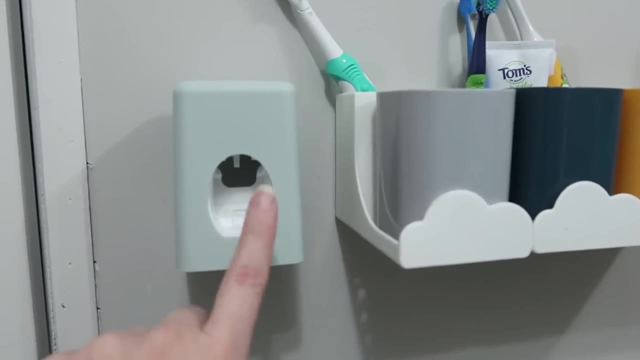 But The heads of their toothbrushes aren't quite small enough. I think Ray's is, but the boys are not- So I just put them up here at the top And then this is actually a toothpaste dispenser, But you got to have the squeeze tube, and the toothpaste that they're using right now is not the squeeze kind. 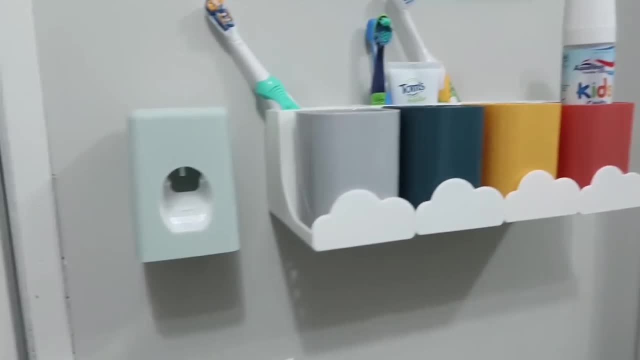 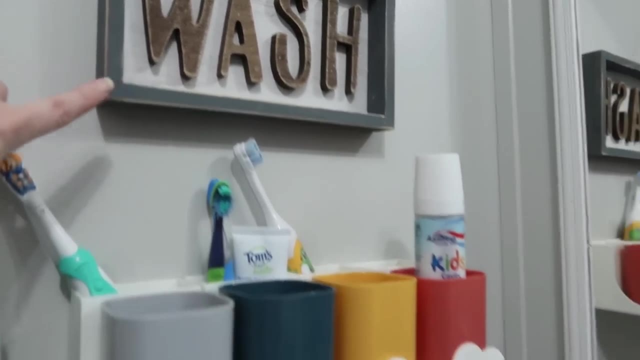 So when they run out of this, I'll get them the squeeze kind that they can put in there and it'll dispense their toothpaste for them. So cute. And then I just took this wash sign that was on the counter Taking up space, and 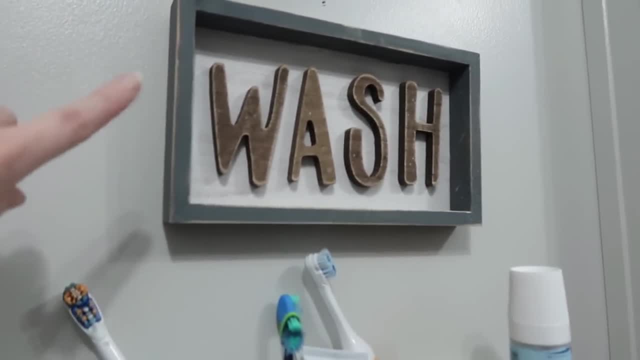 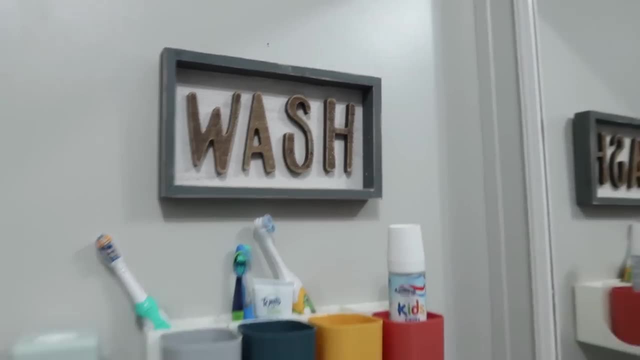 Hung it up here. It worked out perfect because there were actually screws in the wall. They're still there from that other shelf that I had hanging up here, And so this way it hid the screws and it's perfect and it's up off the counter. 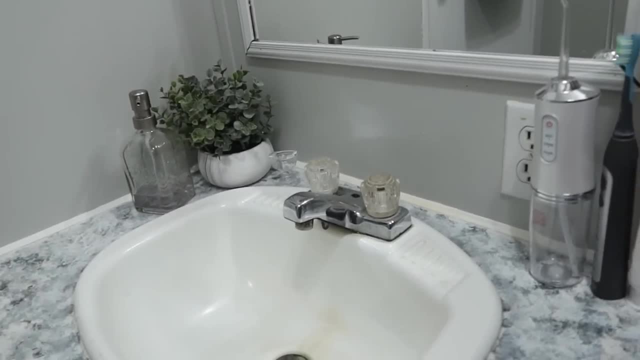 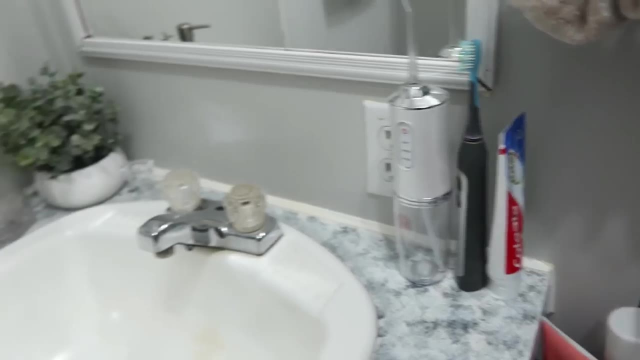 So now on the counter it looks so much better. We don't have near as much clutter. I do still have my toothbrush and toothpaste and my Waterpik sitting there, But over here I just have this piece of greenery: some soap. 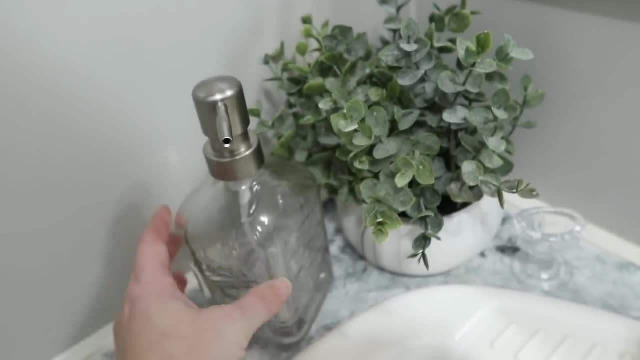 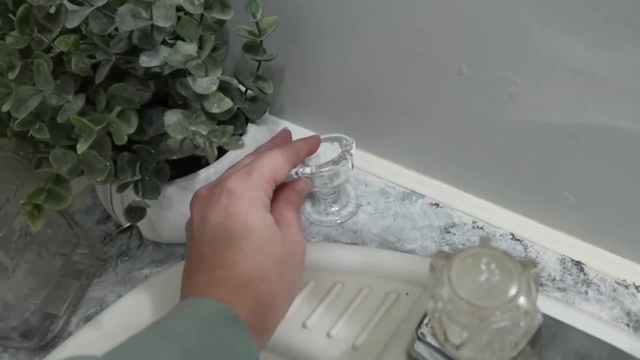 This is just a soap. This is a toothpaste dispenser that I got from TJ Maxx and I poured a piece of bottle of antibacterial soap into. This is an eyewash glass. just keep that sitting there. It's more decorative than anything. 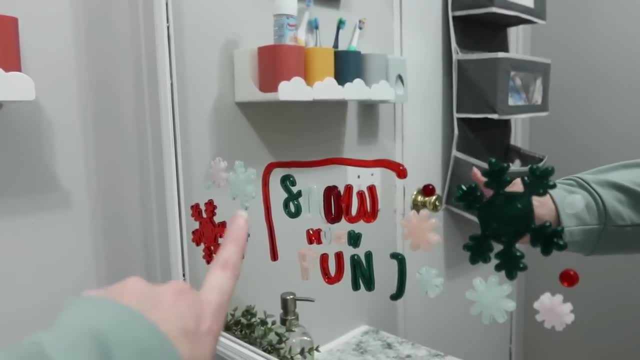 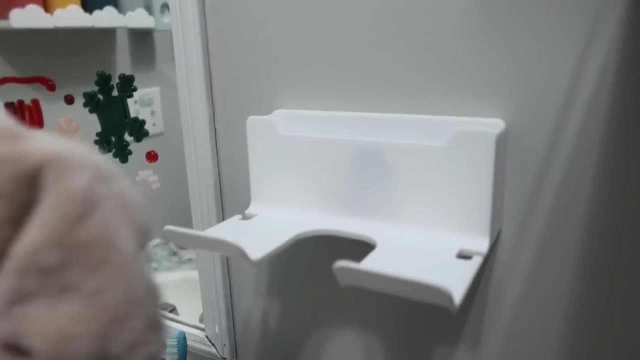 I don't really use it a whole lot. And then this window cling. I think I got from the Dollar Tree. It says snow, much fun, So I thought the kids would enjoy that for Christmas time. And then this is my blow dryer holder, which I'll be using sometimes. 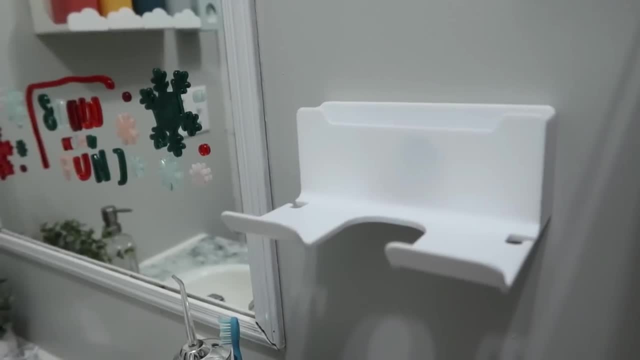 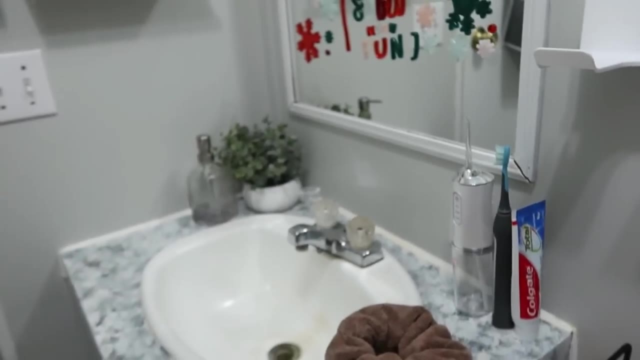 But for the majority of the time I would like my blow dryer To be stored under the sink and out of the way, But there are times when I'm getting ready I have my blow dryer out and all of my things here on the counter. 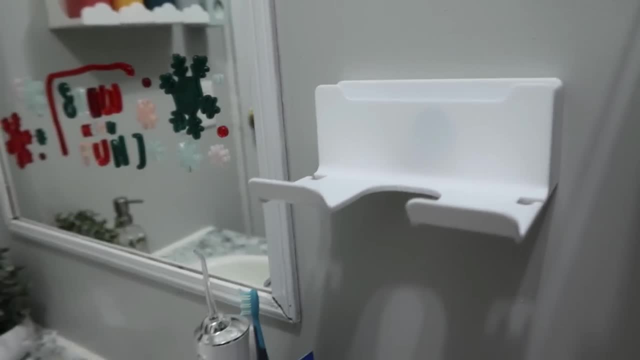 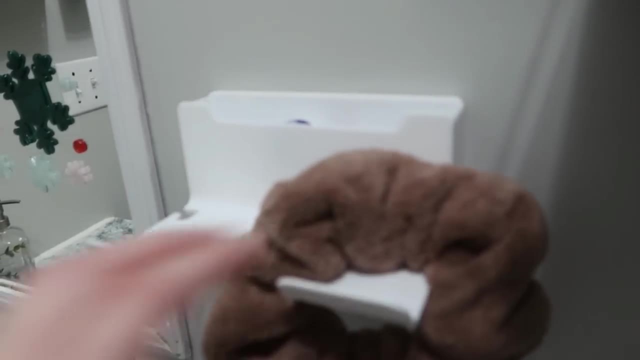 So this will be nice to be able to just hang my blow dryer up and get it out of the way. For now, I have my current contact case that I'm using and some of my towel scrunchies that I use for when I wash my hair. 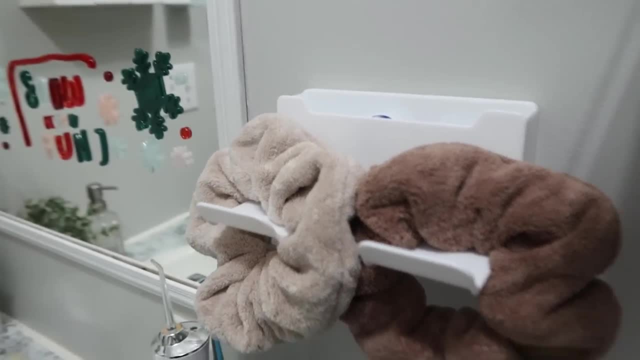 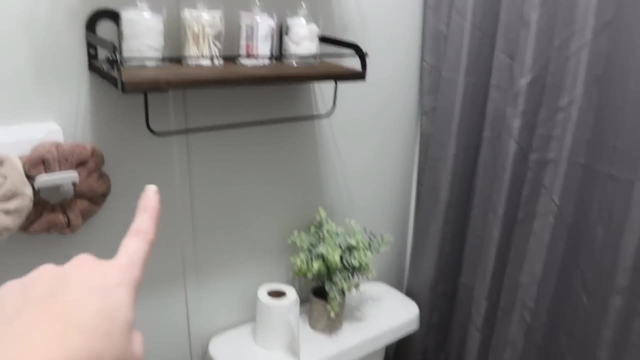 So after you wash your hair, you'll put them up in these, and it absorbs a lot of the moisture from your hair, So I just hung those there Now moving on to my hair dryer. So I'm going to move on to the shelves that I have here above the toilet. 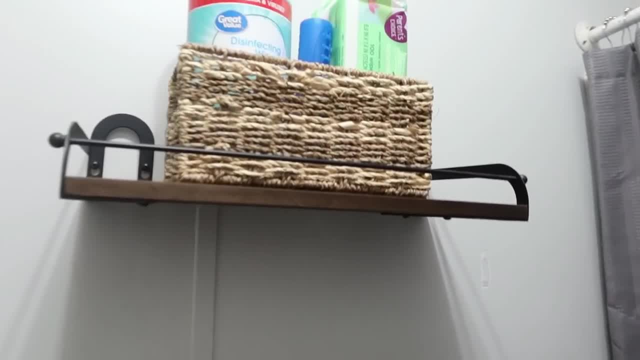 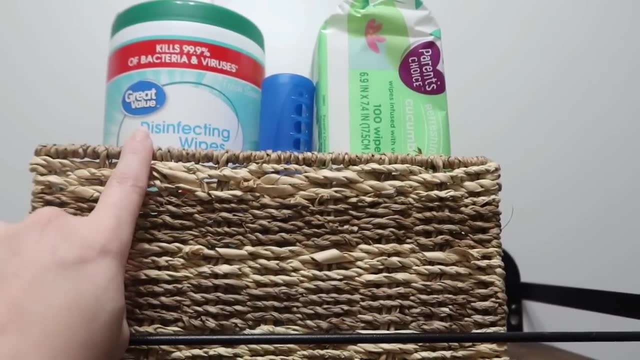 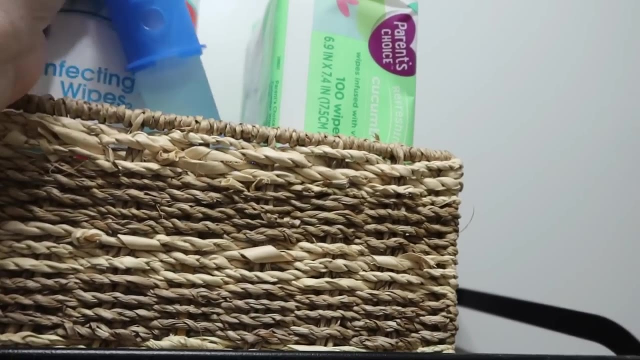 So they are very clean and minimal. now I'm very happy with them Up here in this basket. I just have some disinfecting wipes. I always like to keep a bottle of disinfecting wipes in the bathroom: Some baby wipes because we are potty training, and then this gel stamper for the toilet. 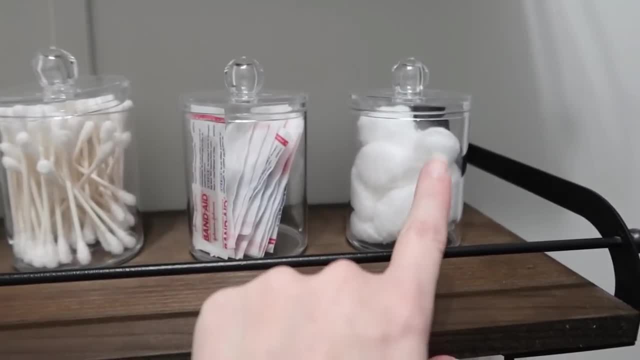 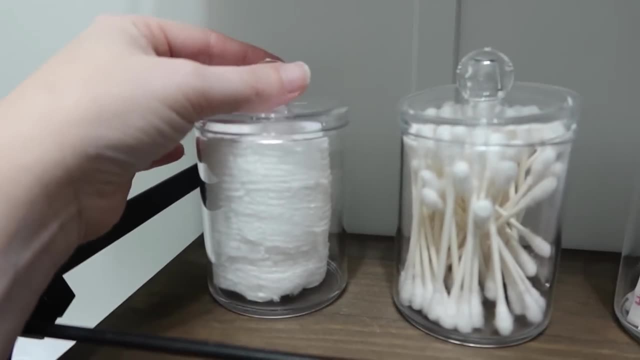 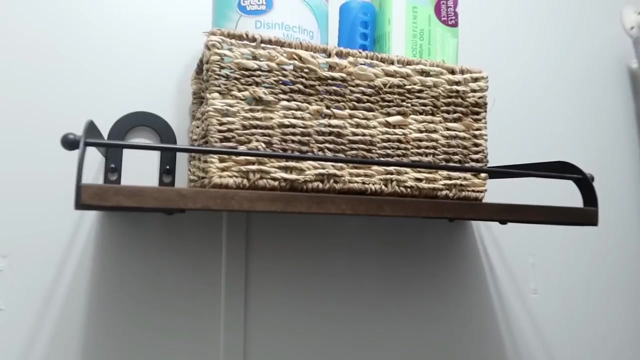 Then down here on this shelf, I love these little jars, So I have some cotton balls, band-aids, some Q-tips And then just some cotton rounds that I use for taking off eye makeup and nail polish. But yeah, I love this shelf and how clean and minimal it looks now. 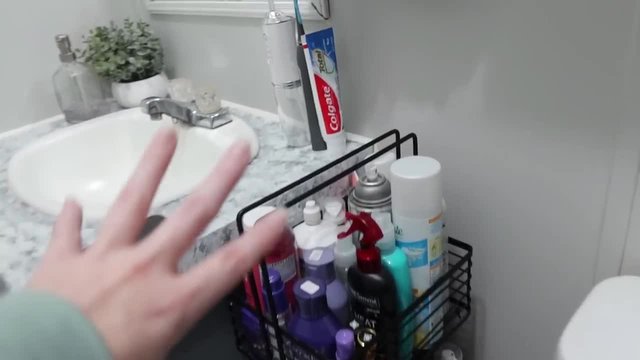 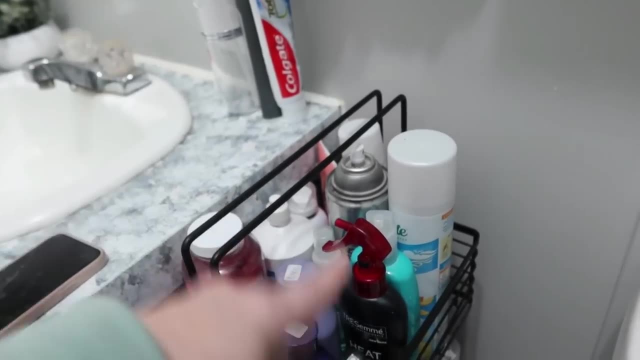 Right here by the sink. I keep all of my hair products up on the top shelf that I grab for the most when I'm getting ready. So things like dry shampoo, hairspray, heat protectant- I've got some detangler. Things like that are on this shelf. 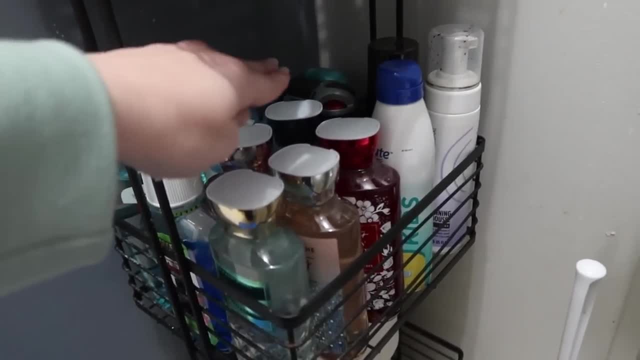 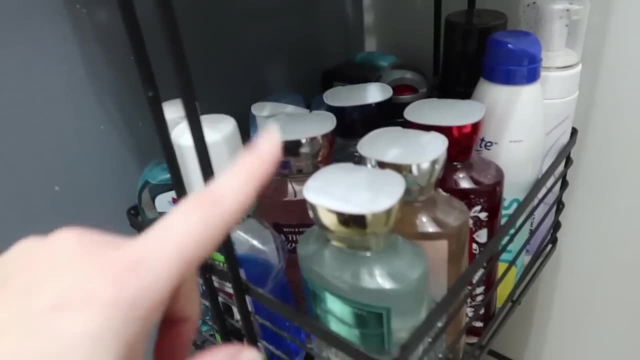 Then on the second shelf I have a few of these things. here i have a lot of extras. so in the back i've got extra deodorant, i've got some extra self tanner, some sunscreen for the summertime, and then recently i went to a bath and body works and 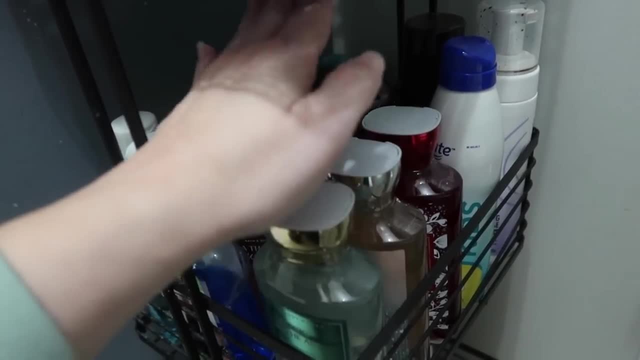 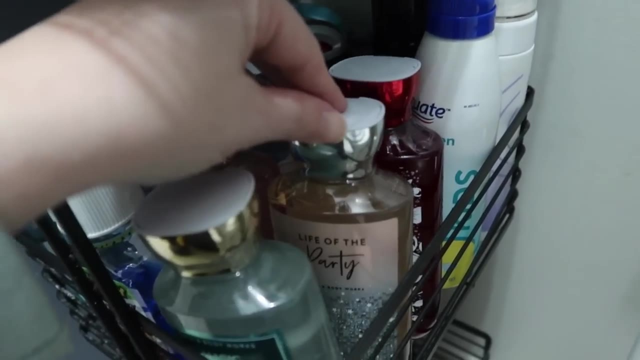 got a few extra body washes to have on hand. i love their body wash and i only get them twice a year when they're on sale, so i went ahead and got a few. so i just got magic in the air life of the party. this one smells amazing. it's one of my new favorites. it's the winter. 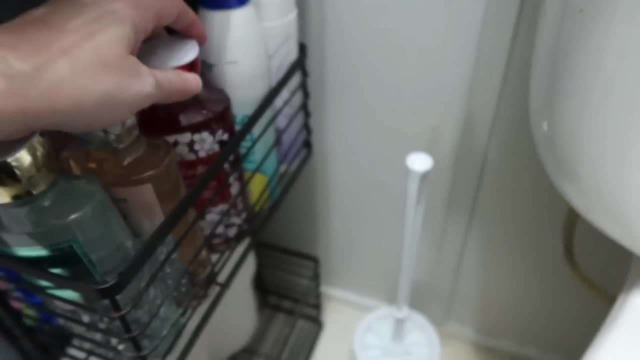 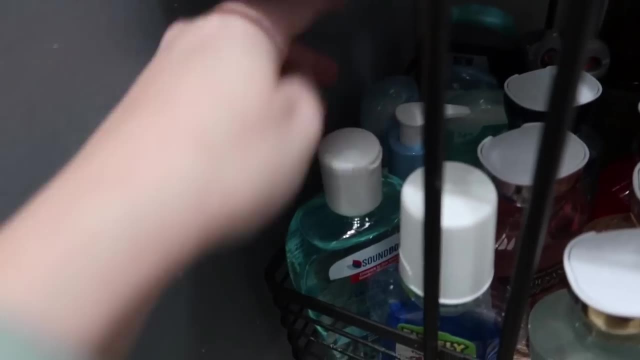 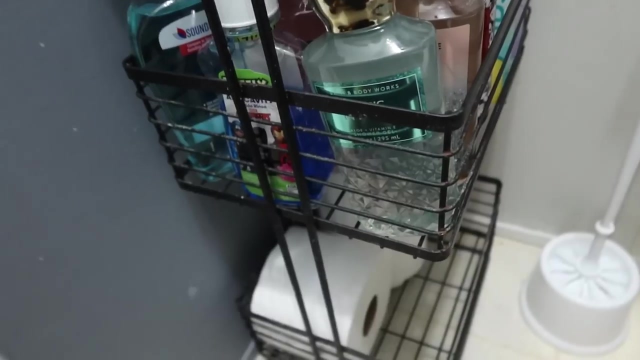 cherry blossom and i got a few to hand out for gifts as well. and then i got gingham- y'all know that's my favorite- and a thousand wishes. i have like extra face wash and some astringent, and then down here on the bottom i just have extra toilet paper that wouldn't fit in the over the door. 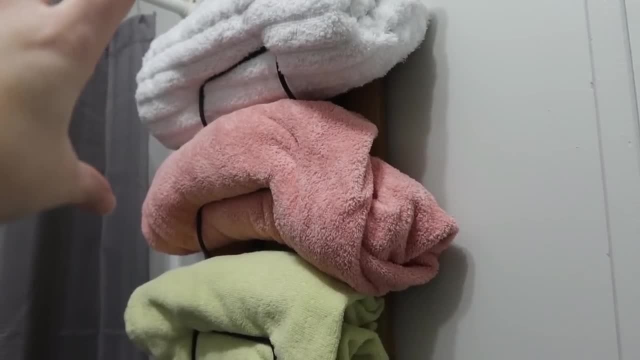 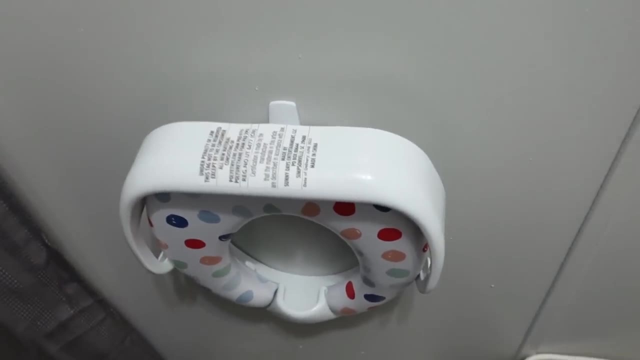 organizer. and then i also fixed our towel rack where it's not halfway hanging off the wall now. so i got that fixed and restocked us with towels. and then this: i decided for ray's potty training just to take her other potty chair to her dad's house and she can use. 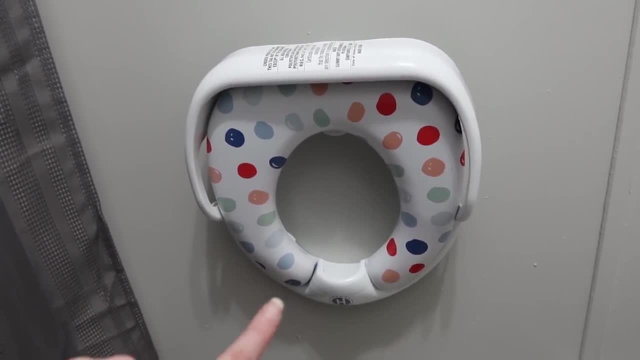 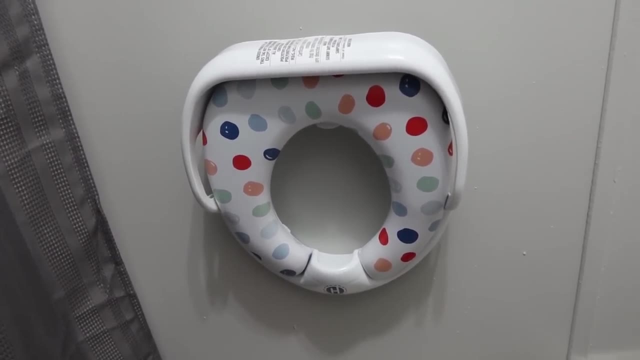 it there. but this is going to be the easiest because you can just set it on the toilet and flush when she's done, versus having to clean the toilet seat every time she uses it. so i'm just going to take her other one to her dad's, and i got this one from walmart. it was really 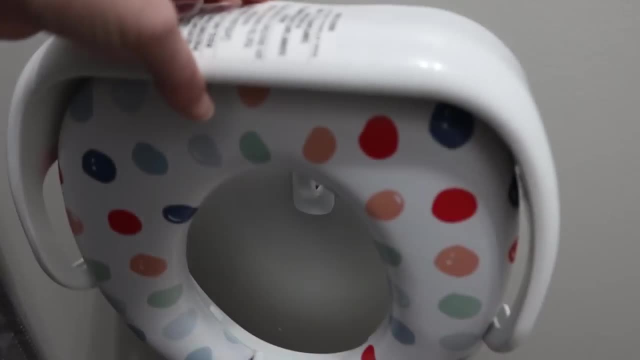 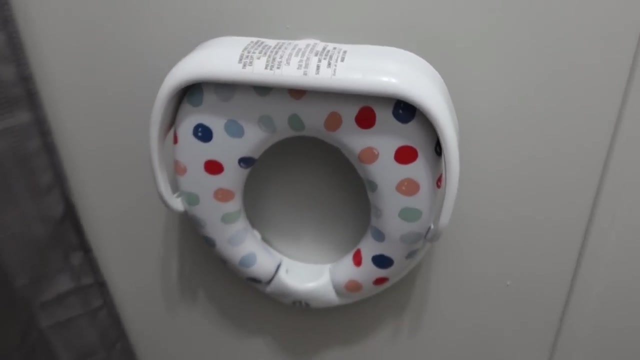 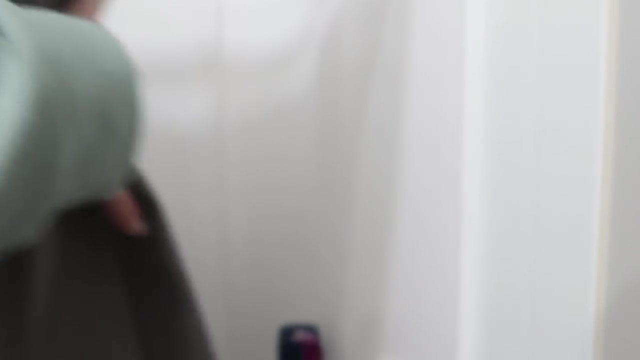 inexpensive, and i just hung it up with a command hook. it does come with a hook to hang on the side of the toilet, but it wasn't going to work out there. we just don't have enough room to hang it there, so i just used a command hook and hung it there for now, so, and then into the shower. 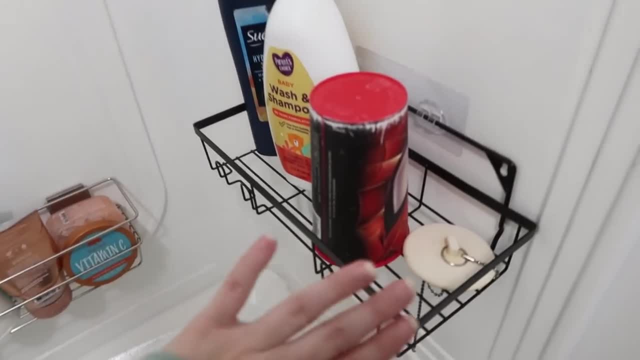 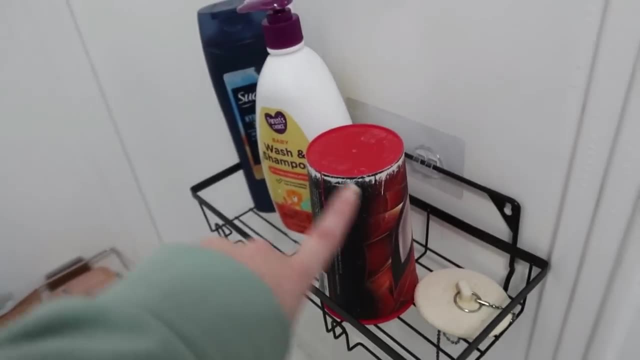 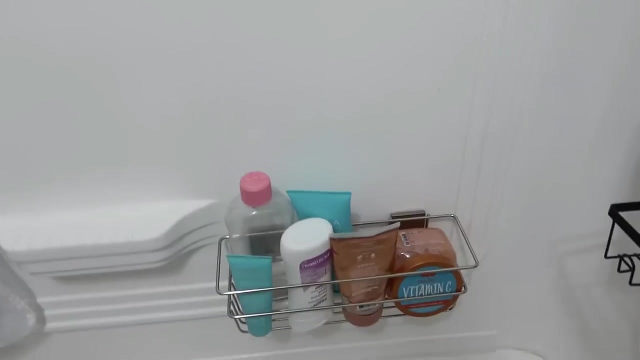 so i got this hung and this cleared up all the extra things that we had sitting on the edges of the tub. so we got the cup, the plug, um, some baby wash, and then kai's body wash there, and then that's just all of my products that i keep there, and then i'm just going to hang it up with a 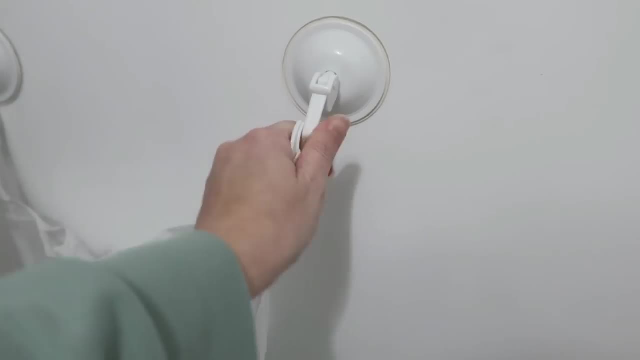 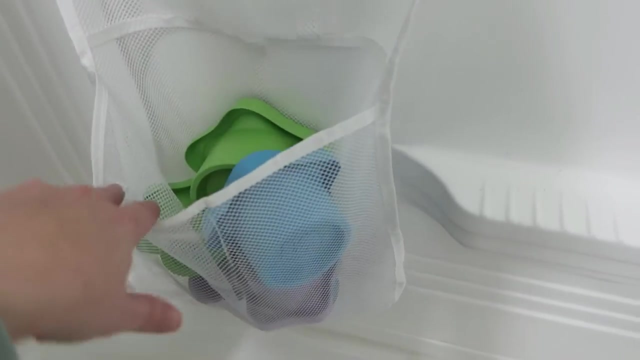 and then this net was super easy to hang. so to suction it you just flip the hooks down, and then to unsuction, you just lift them up and it comes right off, and then to resuction you just flip it back down. but this will hold all of her bath toys. she loves these little stackable cups. i got those. 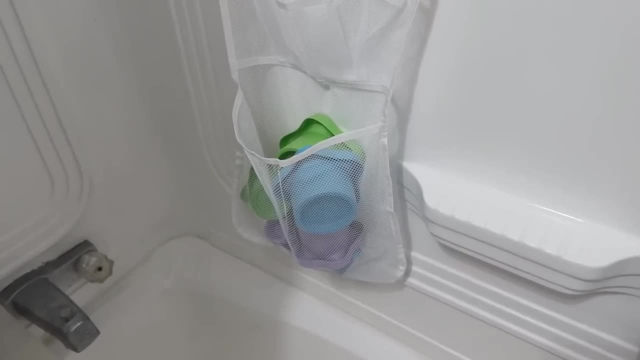 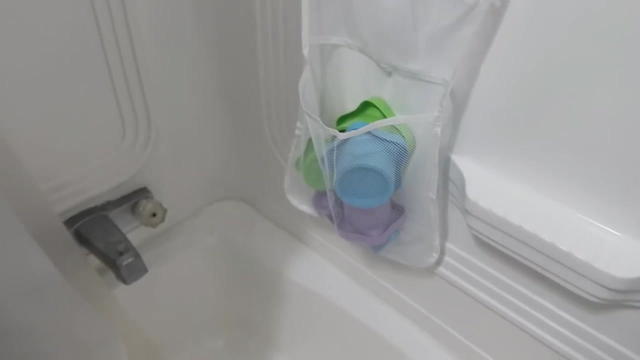 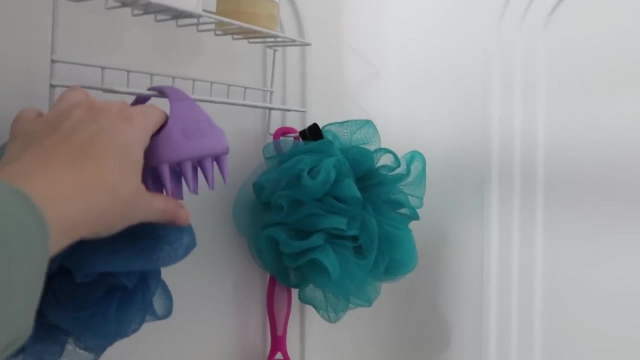 from walmart. i really don't like those bath toys that hold water. i like the kind that i can wash if i need to and get nice and clean. so there's all of her toys here. i just decided to keep everything up here how it was. so i just have my shampoo and conditioner, my scalp massager. 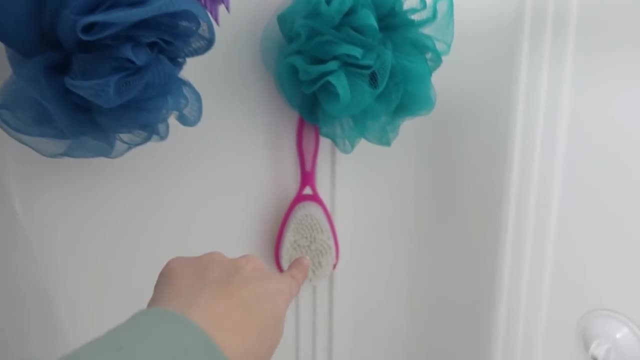 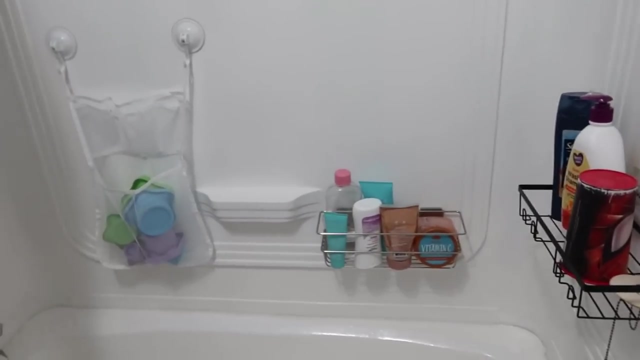 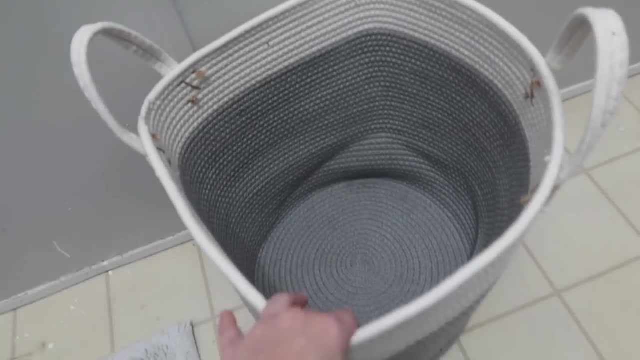 for when i wash my hair and our loofahs, and then my back brush that i like to use. but yeah, that's all for the bathtub. my main goal here was to get the extras up off the edge of the tub, and this little thing here was perfect. and then down here we just have our new laundry hamper. i love that. 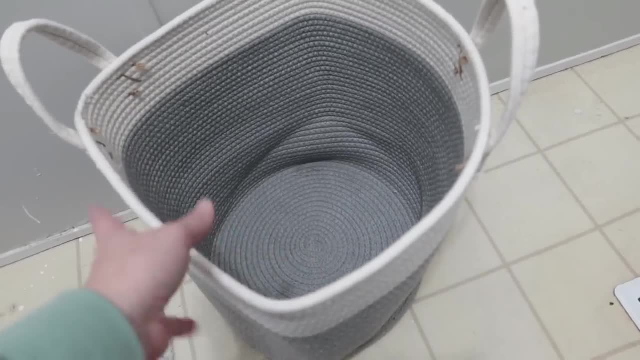 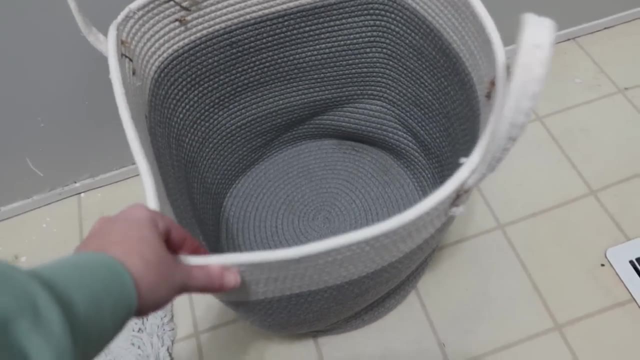 it has handles, so it'll be really easy to pick up and carry to the laundry area. but when we're in here bathing and taking showers, we can just throw our dirty clothes right into this. then, of course, when it gets full, just take it on to the washer. and now 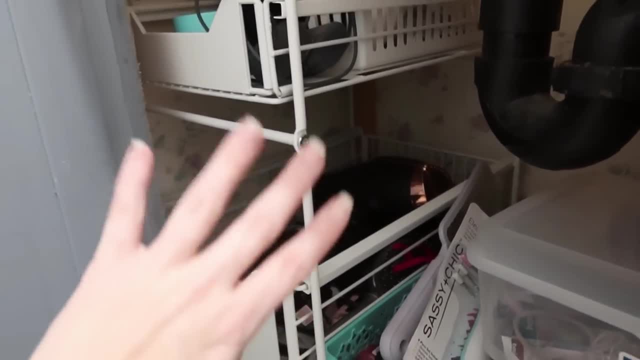 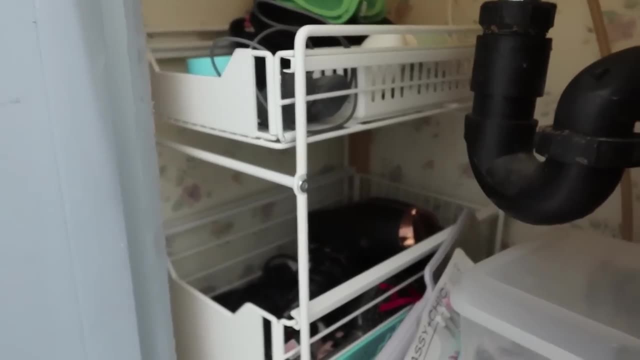 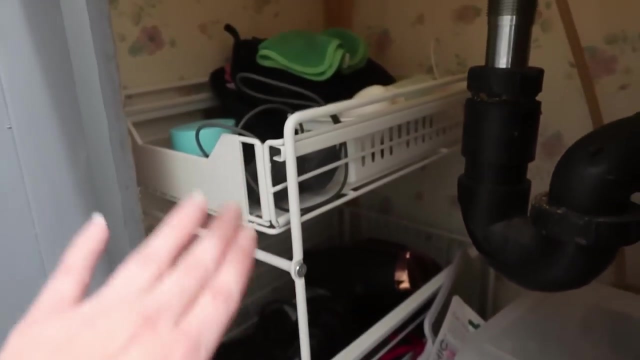 under the sink, so this did not work out like i was hoping it would. it's a little bit too wide, the way that our pipes are. i actually had to take it apart and reassemble it where i wanted it to sit. i can't use the drawers, but it's fine because it still holds my stuff and i'm 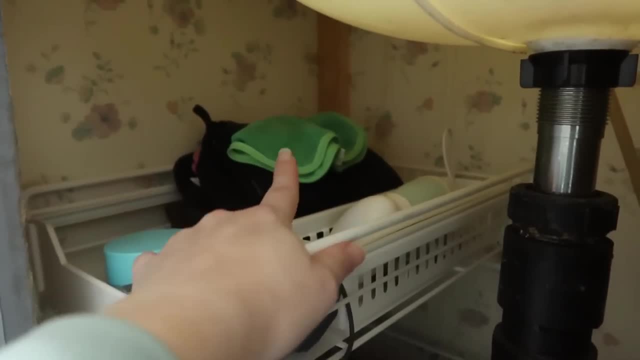 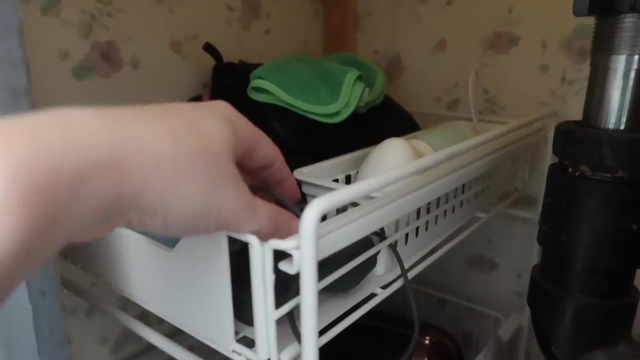 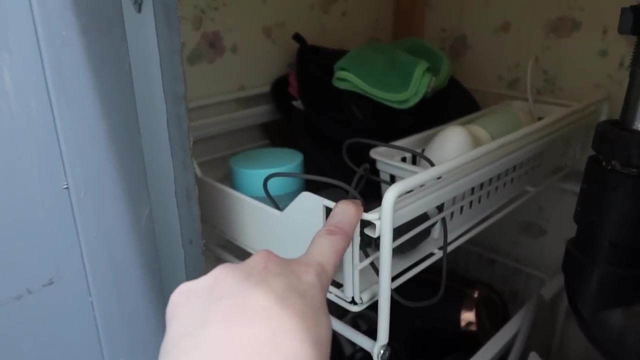 able to access my stuff. so up there i just have my makeup remover cloths, my face washing brush and all of its accessories are in that basket- my toothbrush charger. i decided to put that up because i very rarely have to charge my toothbrush- it's like once every six months- so i just decided. 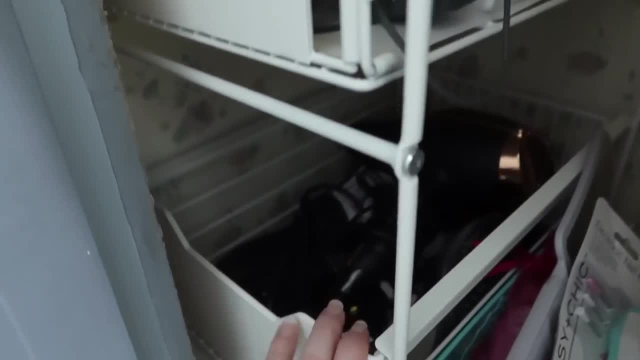 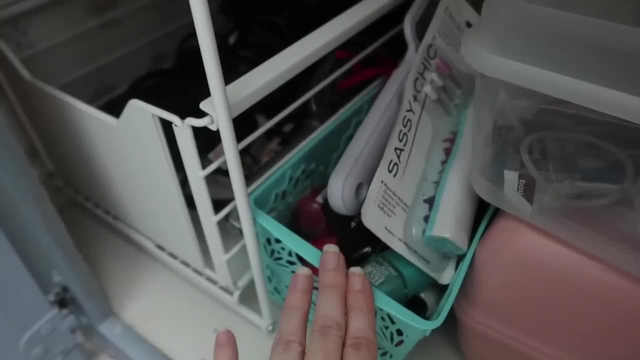 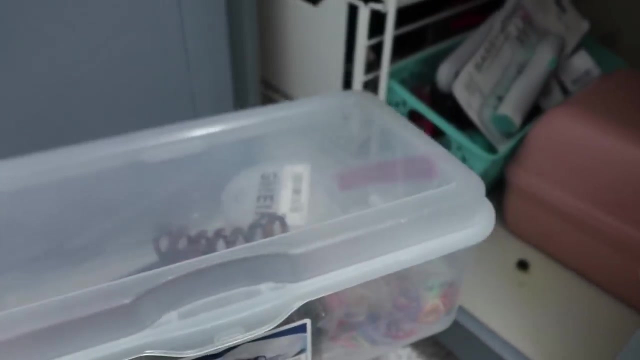 to put that away, and i've got my face cream there, and then down here i have all of my hair tools stuff here. i decided to put all of our hair things, so i've got hair clips, hair ties, things like that in here, and then right over here i just have my caboodle box. this holds all of my makeup, but that. 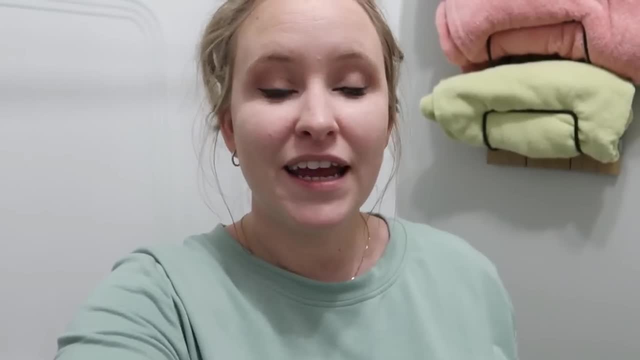 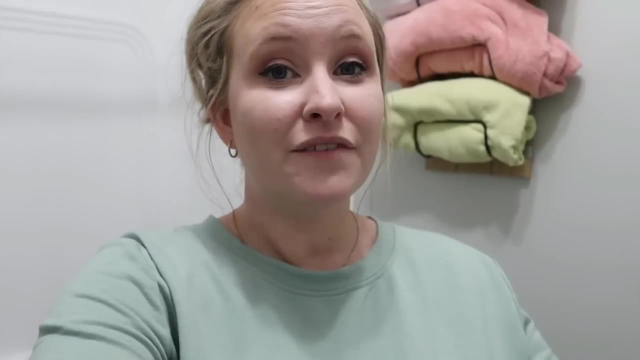 is gonna do it for today's video. i really hope you guys enjoyed and got some motivation to declutter and organize whatever space you are working on in your own home. if you're still watching, make sure to leave a butterfly emoji in the comments down below and also a. 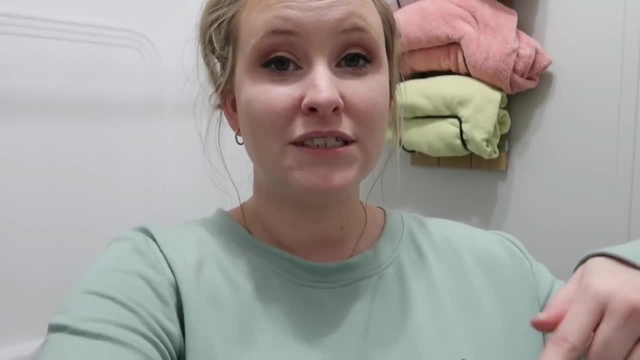 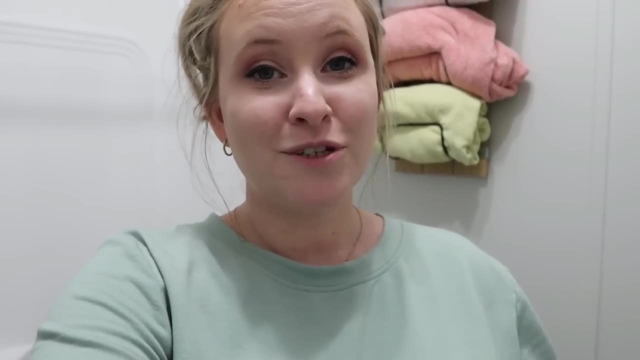 thumbs up because it does help me out a ton. and remember, if you want to download and shop the tmoo app, i'm gonna have that link and discount information in the description box down below. thank you guys, so much for watching and i'll see you in the next one. bye. 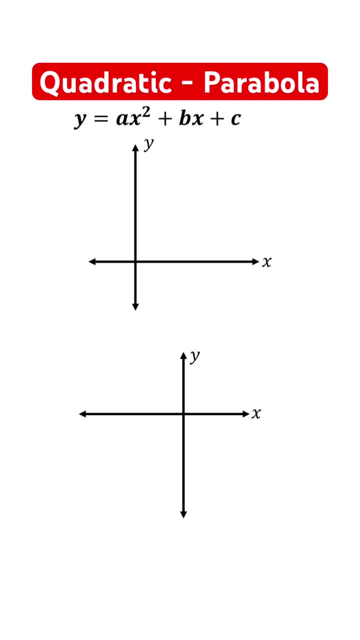 The graph of a quadratic equation is U-shaped curve, called a parabola. When the leading coefficient is greater than zero, the parabola opens upward. When it is less than zero, the parabola opens downwards. The vertical line that divides the parabola into two equal halves. 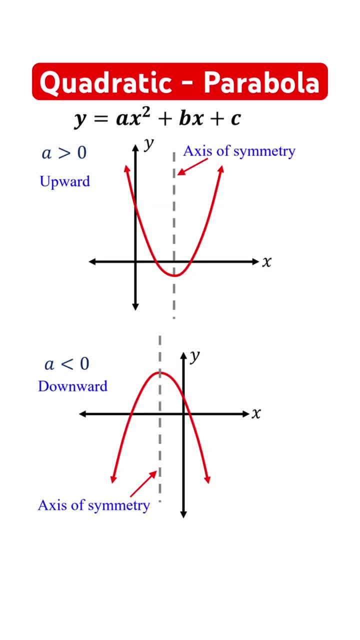 and passes through its center is called the axis of symmetry. The turning point of a parabola is known as the vertex. The vertex always lies on the axis of symmetry. If the parabola opens upward, the vertex is its minimum point. 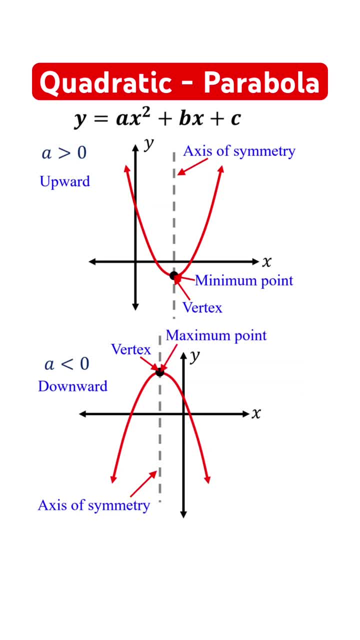 If it opens downward, the vertex is its maximum point. The point where the parabola intersects the y-axis is called the y-intercept. It occurs when x equals zero. The points where the parabola intersects the x-axis are its x-intercepts or roots.